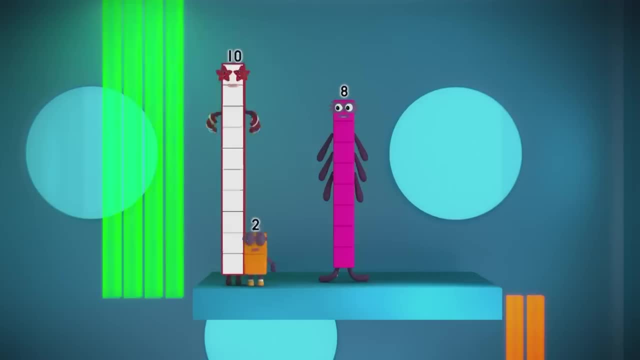 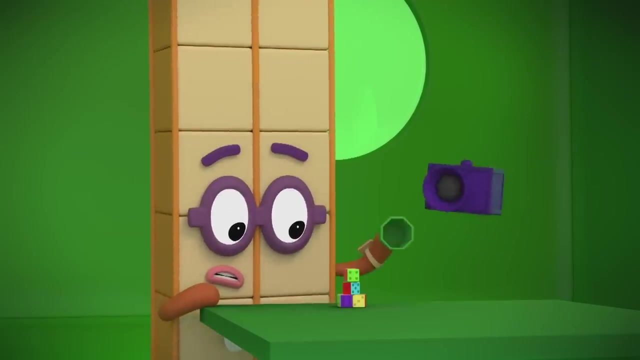 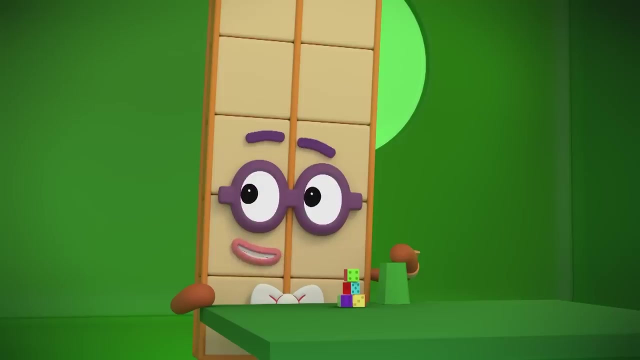 Eighteen and two, Aww Twelve and eight. Switch Four by three. Whee, Ride the rays Up and away. You'll find four dice inside this cup. Roll four fours, then climb on up Four fours. I'd need to be the luckiest number in Numberland. 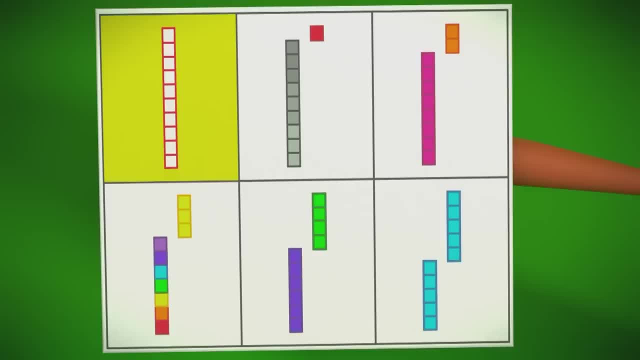 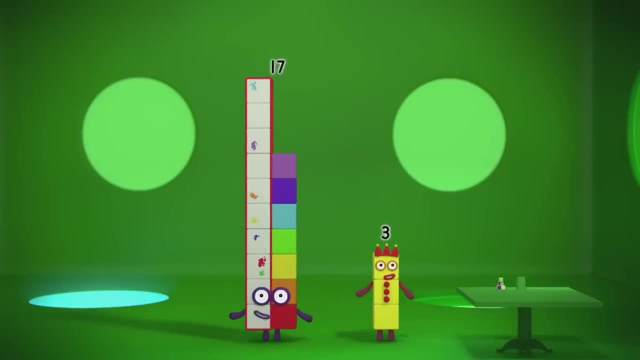 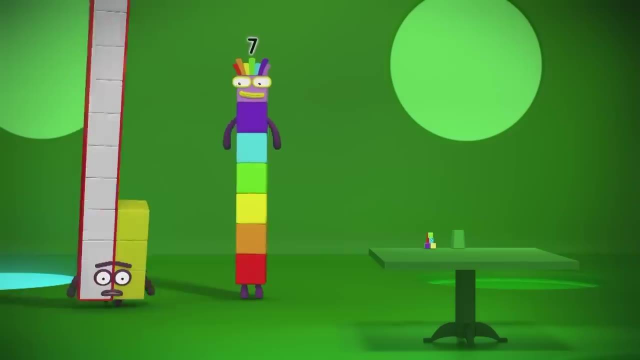 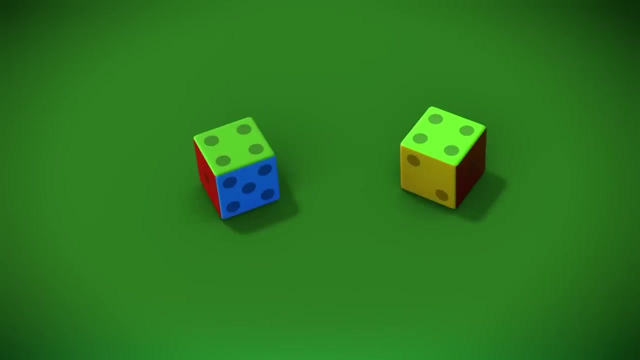 Four by three, Four by three, Four by three, Sixteen and three Or thirteen- Oh, don't say it, I think this is more your sort of thing. Seven- Pretend I'm not here- Four, Four, Four. 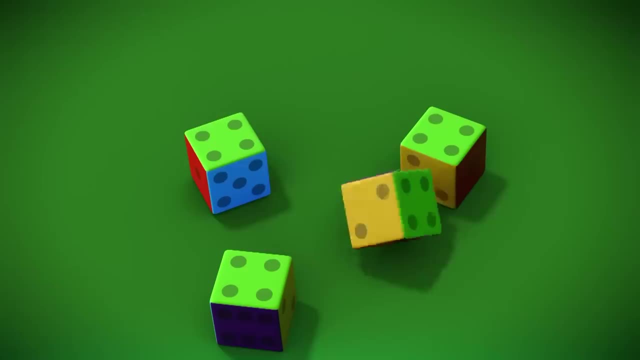 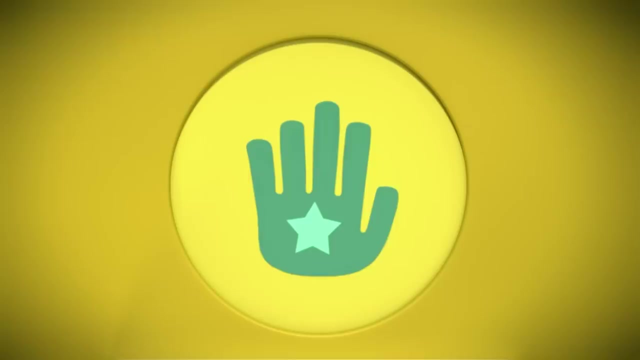 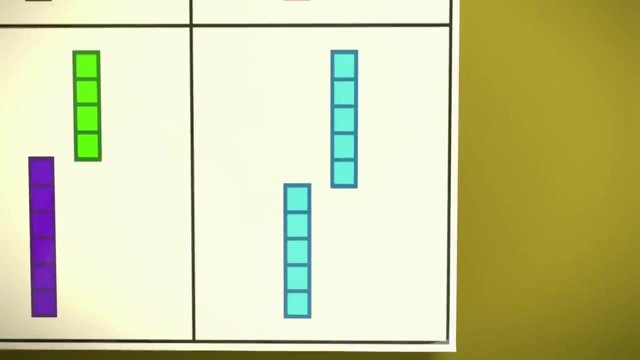 And One more, Oh Oops, Oh, Thirteen, Whee, Wahoo. And Two, Four, Four. That was lucky, Let's see. A hand scanner must mean five. So if ten can be five and five, then I can be. 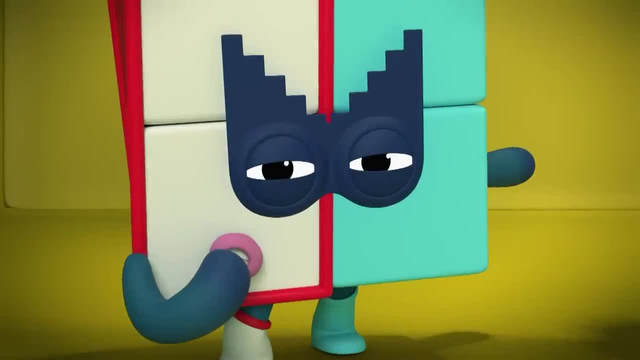 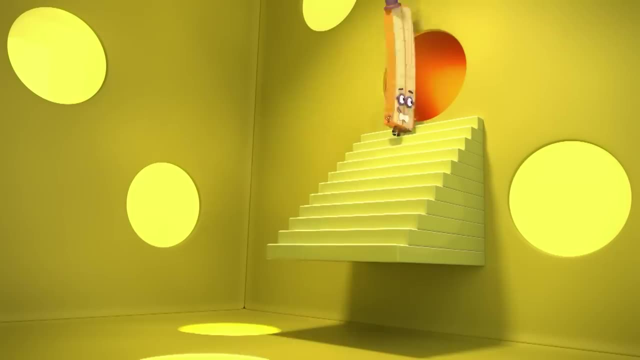 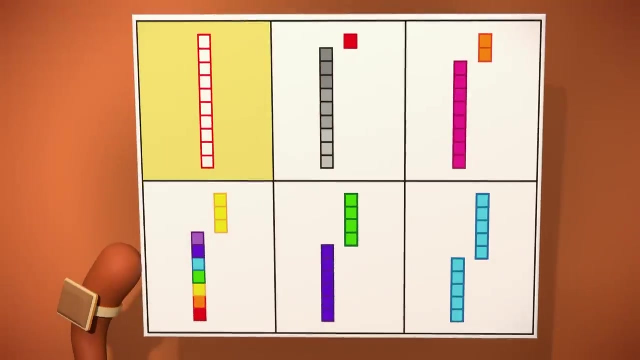 Fifteen and five Hush hush Steps must be taken. High five, Ha-ha-ha, Tip-top. Two high-up buttons to tap, and I know the pair to do it. If ten can make nine and one, then I can make. 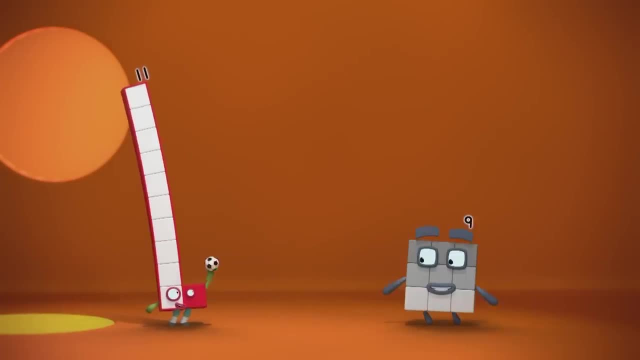 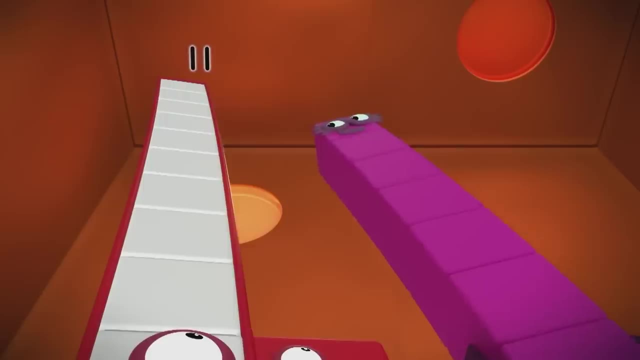 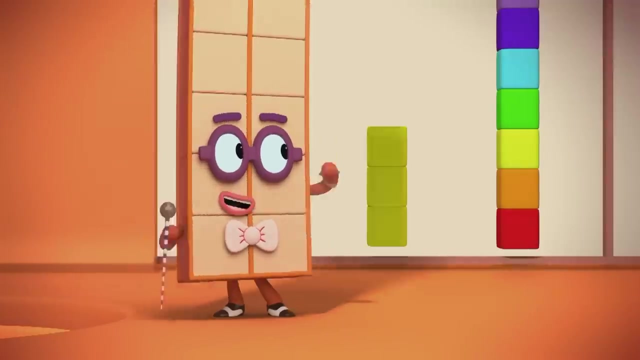 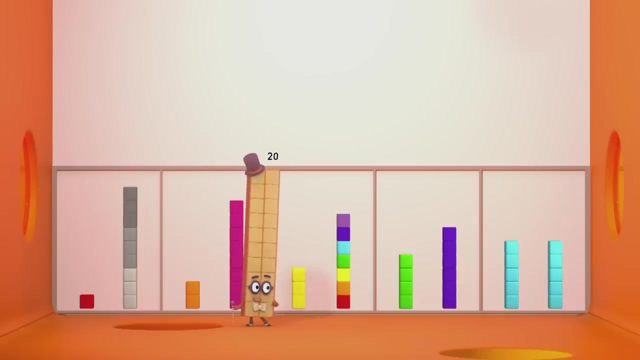 Eleven and nine. Give it your best shot Will do. Yay, Five floors done, One more to get. But can you see the pattern? I can, I can, I'm ten and ten. so my twenty friends are the same as ten's ten friends. 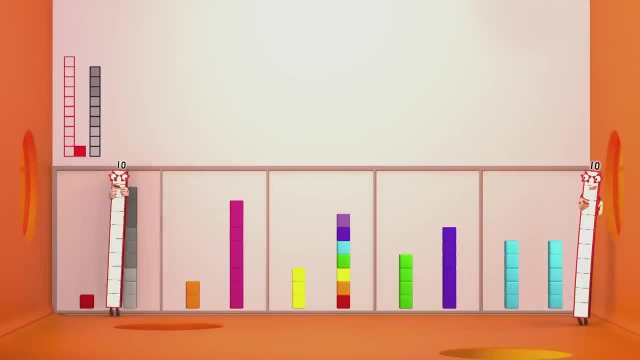 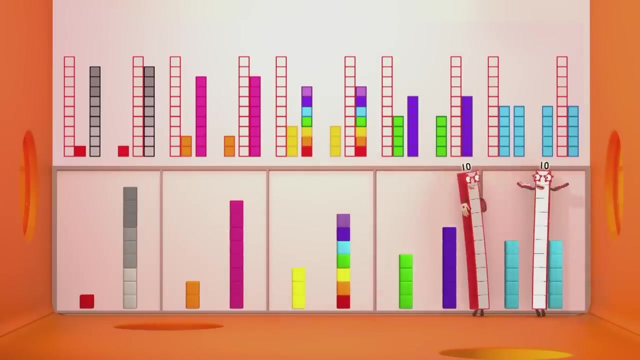 Plus another ten, Eleven and nine or one and nineteen, Twelve and eight or two and eighteen, Thirteen and seven or three and seventeen, Fourteen and six or four and sixteen And fifteen and five, either way round. 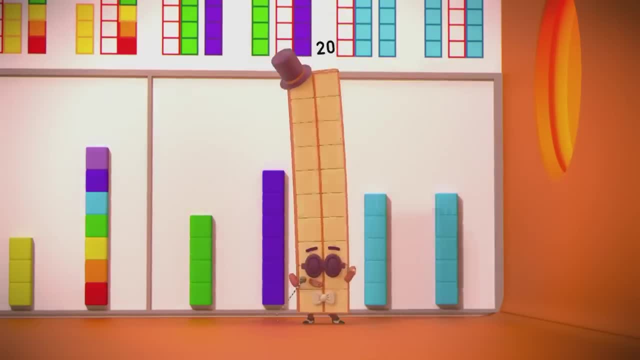 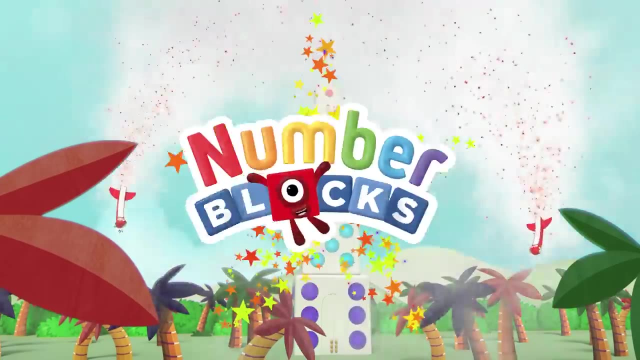 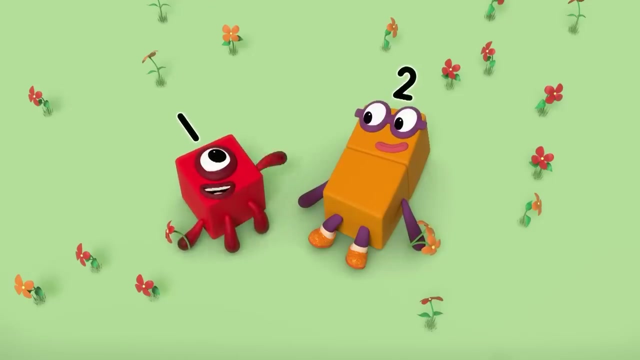 If I'm ten more than ten, then I can make. If I'm ten more than ten, then I can also make. If I'm ten more than ten, then I can also make. Two tens, Two tens Blast off. Oh, it feels like a long time ago. I fell from the sky all on my own. 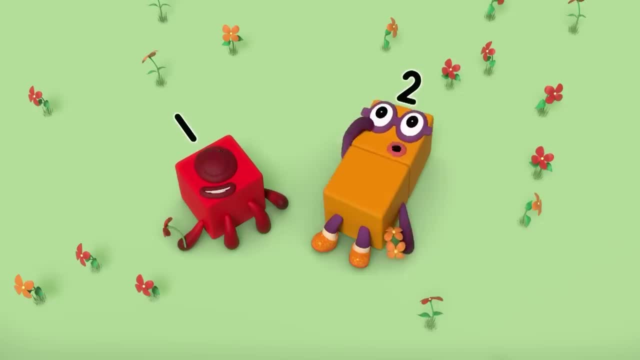 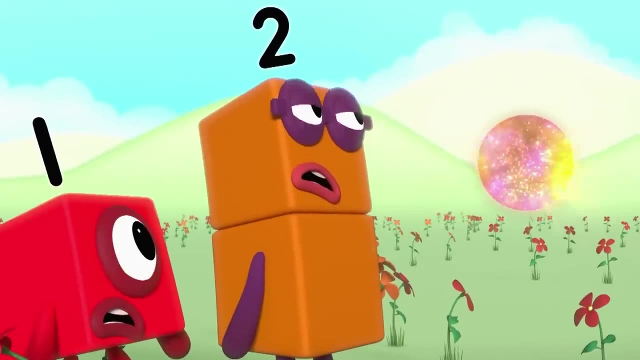 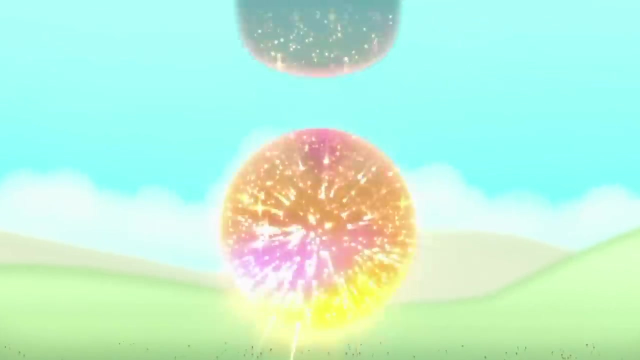 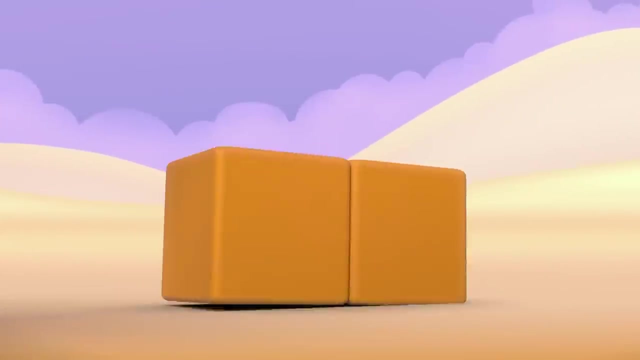 Oh, what was it like being the first? I sometimes wonder: what if I'd been the first number block? Now, that's an interesting question. What? What if two was the first number block? Imagine that. Oh, what's happening. 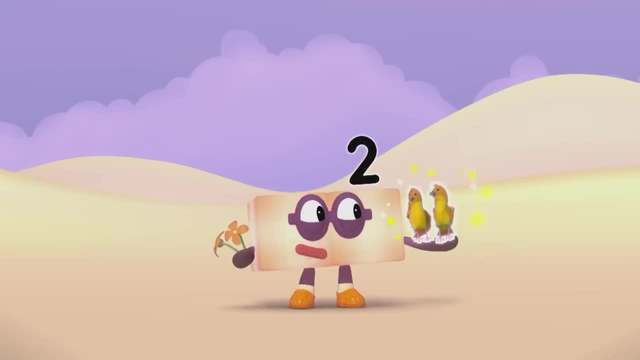 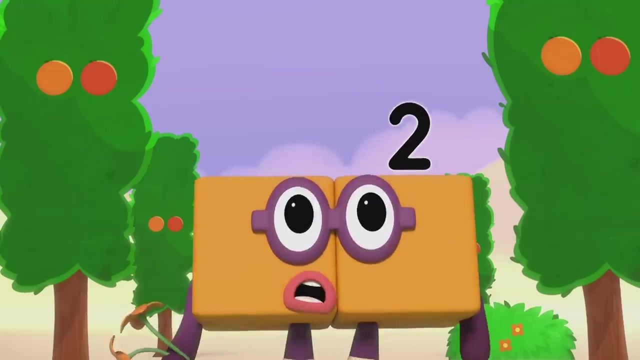 Where am I? Two, Two birds, Hello birds. Boing Boing. Two, Two blobs, Hello blobs. Welcome to Two-Land. Boing Boing. Another falling two. That's two of us. Two, twos are four. 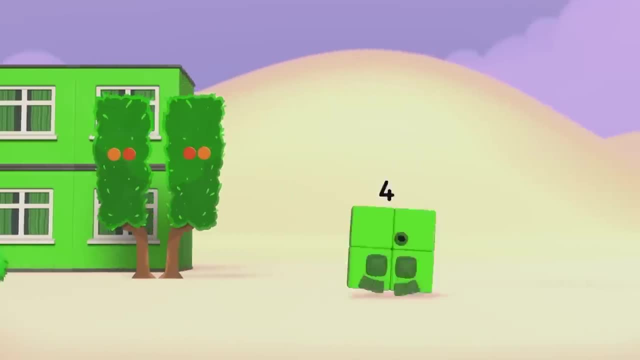 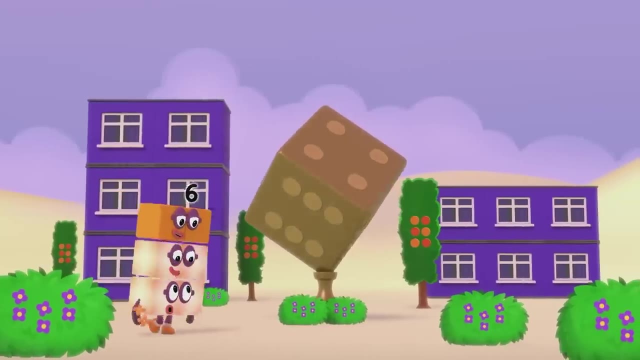 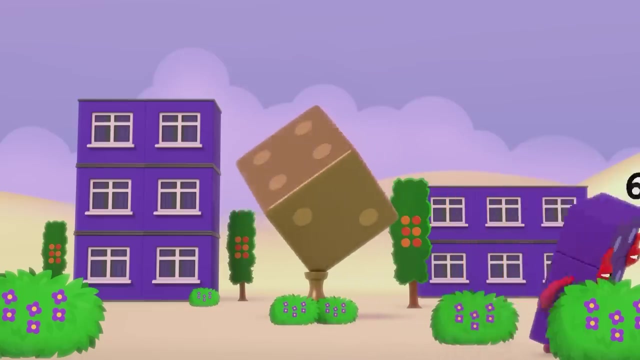 Two, twos make a square, Another two, and now I'm six. Two-Land must be playing tricks. Two, four, six, Only even numbers. How odd, I mean. how even I like this game. I think it's great. 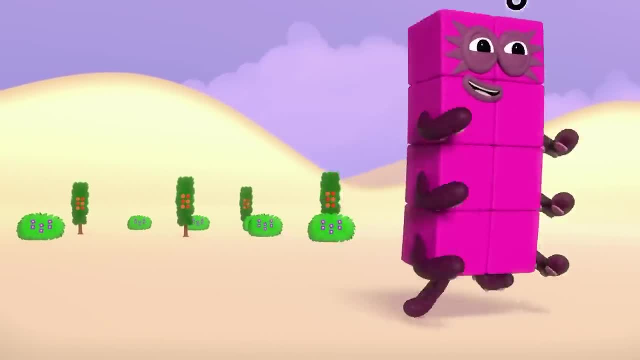 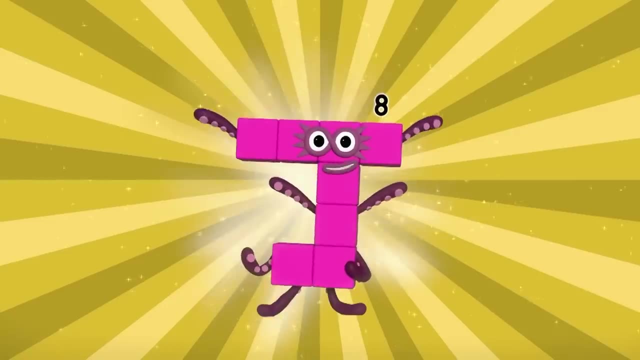 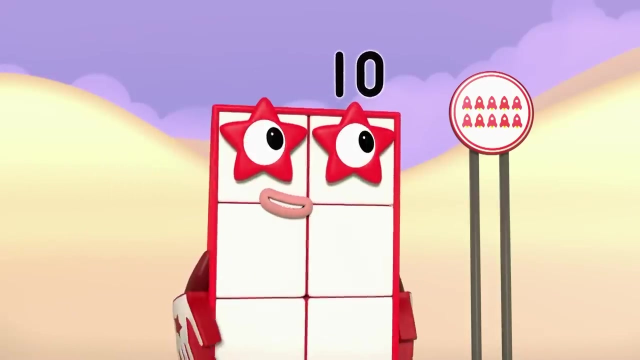 Bye-bye six And hello Eight. Hmm, it's raining. twos: Activate defences, Octoblock umbrella. Two, four, six, eight, Ten. Can some two please tell me what's going on? You're in Two-Land, my friend. 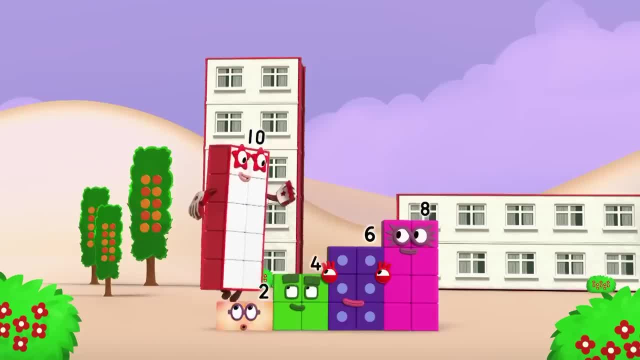 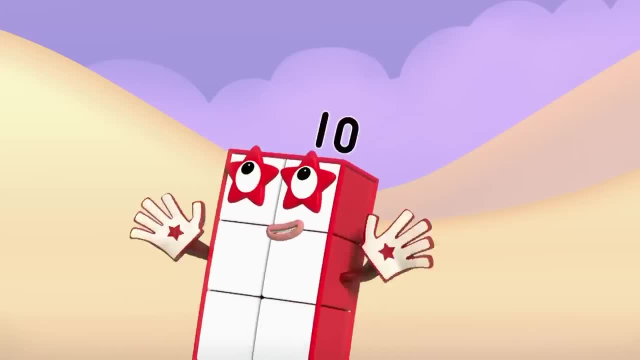 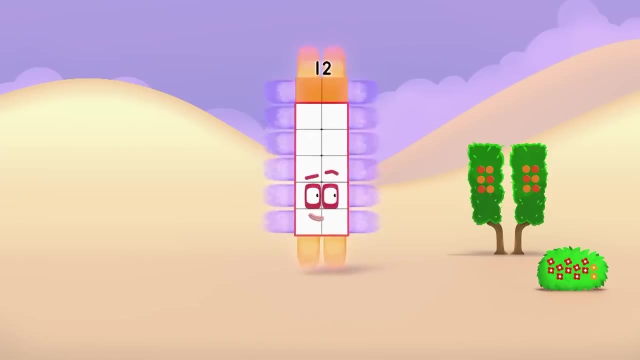 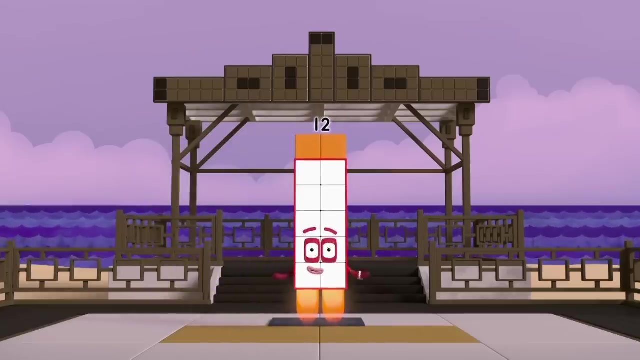 Where every number is Two More Than the number Before: Two, Four, Six, Eight, Ten, Twelve, And I am a super rectangle Two by six. This is where I'm meant to be, For I am. 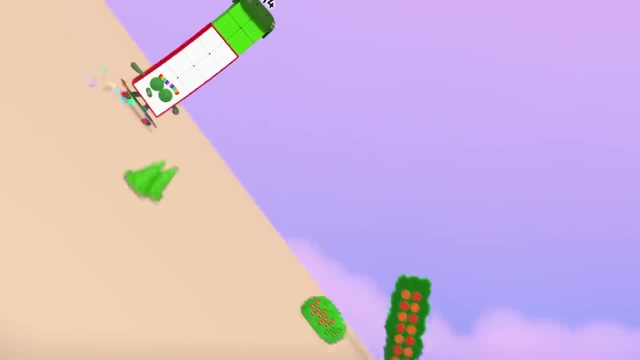 Extreme: Fourteen, Four, Six, Eight, Ten, Twelve, Fourteen, Whoa, Whoa Lucky double, Whoa Lucky double. Ahh Oof, Oh, How odd. I mean how, even No way. 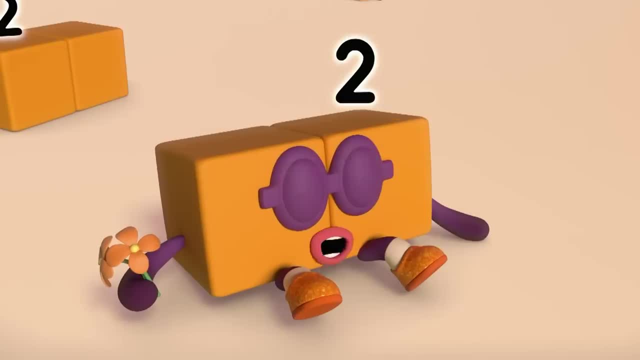 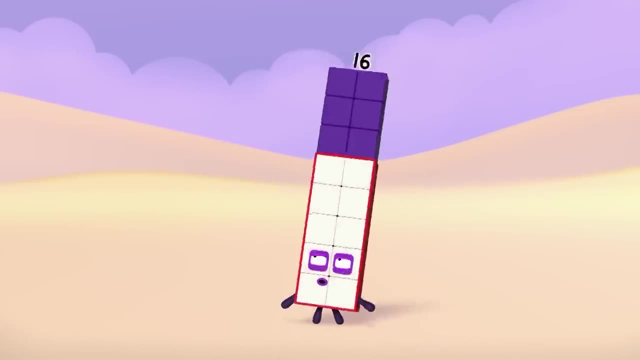 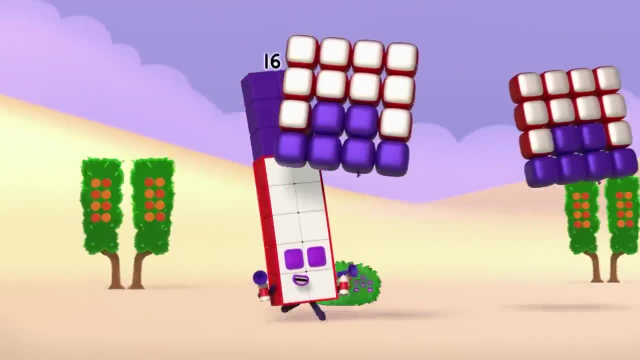 No way I belong in Two-Land too. Pears party, Pears of twos, Pears of fours, Pears of eights. Me again, A square made of pears. Who's next Eighteen on the scene. 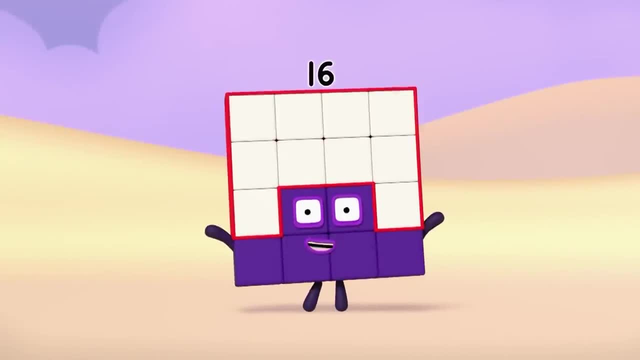 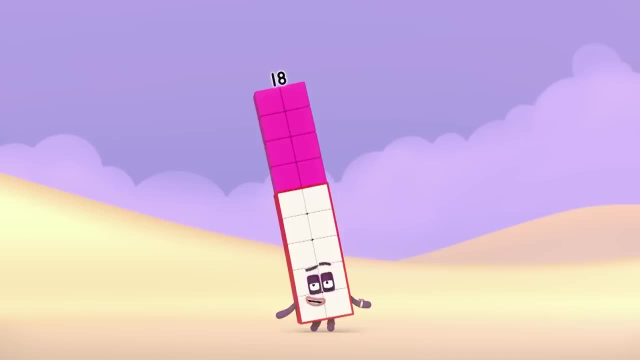 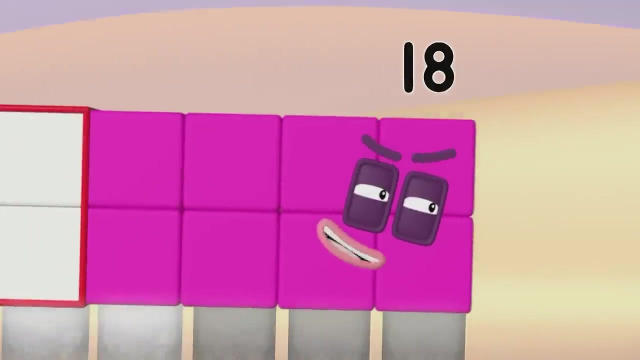 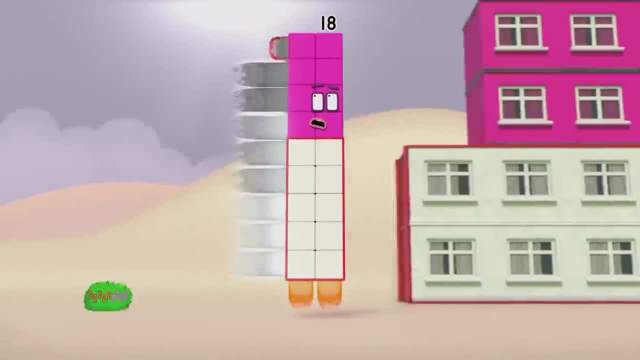 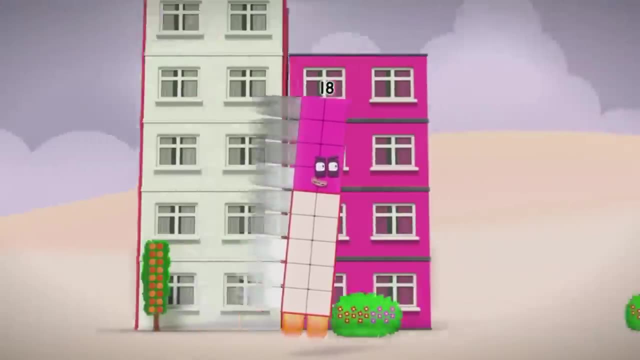 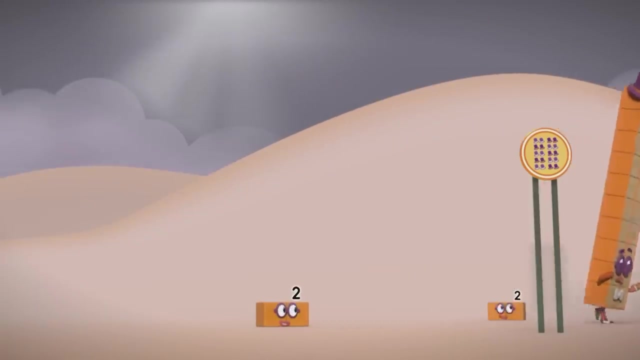 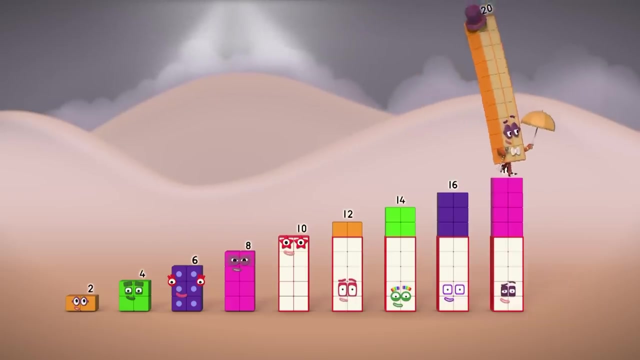 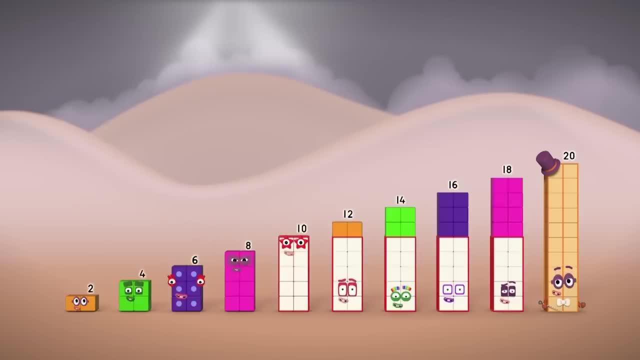 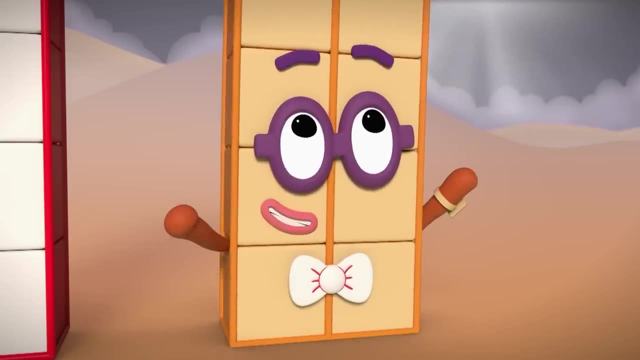 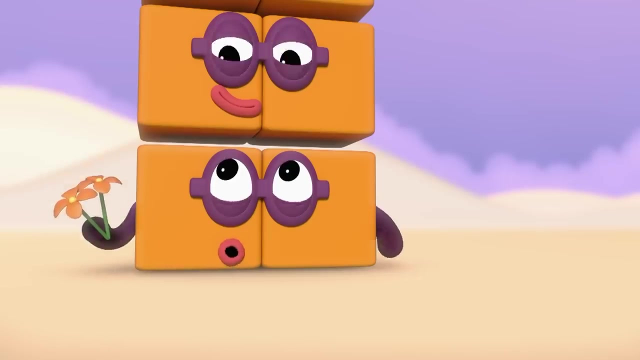 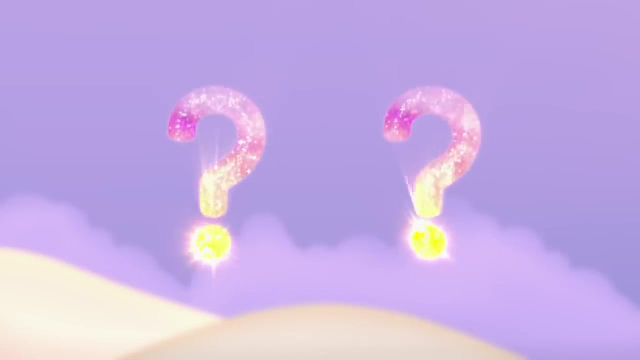 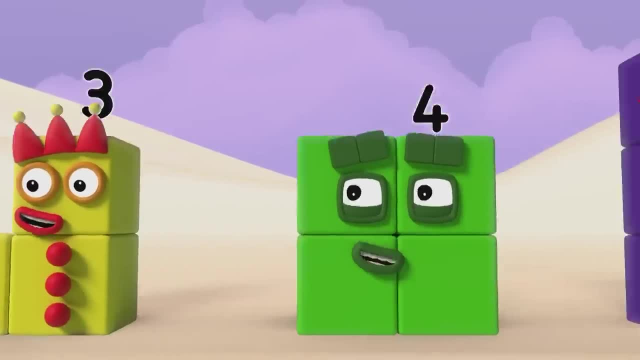 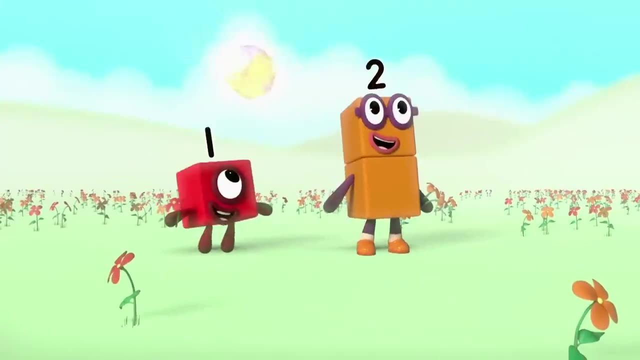 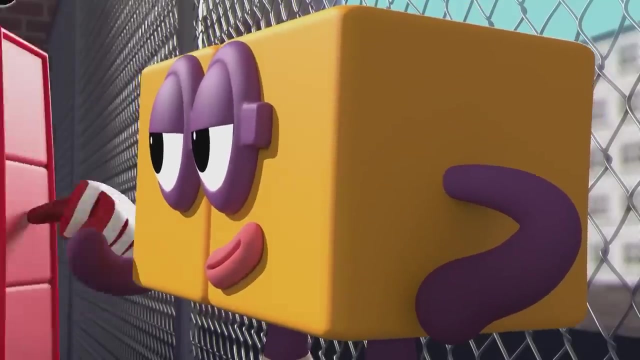 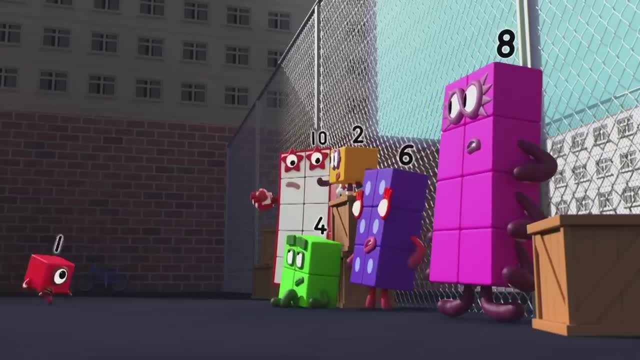 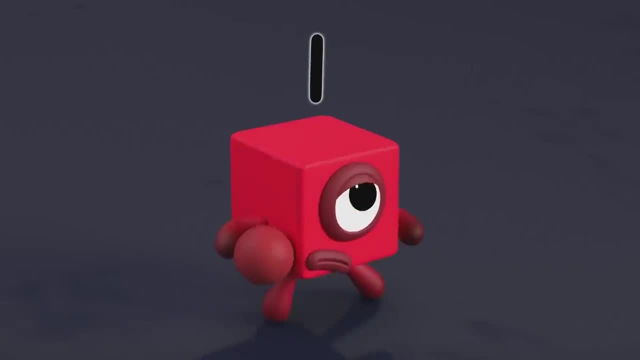 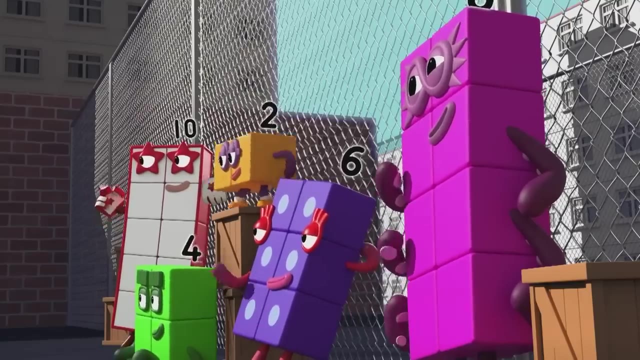 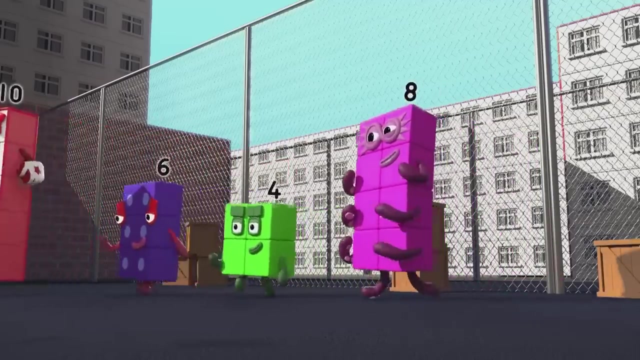 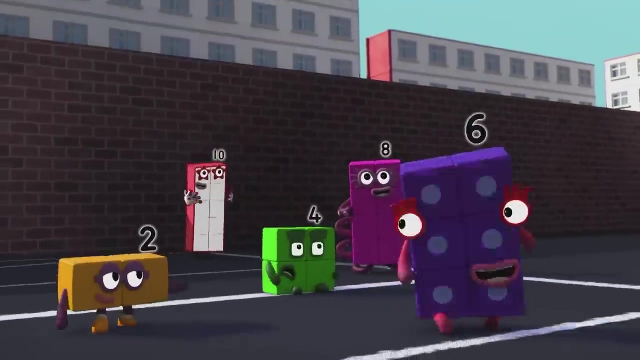 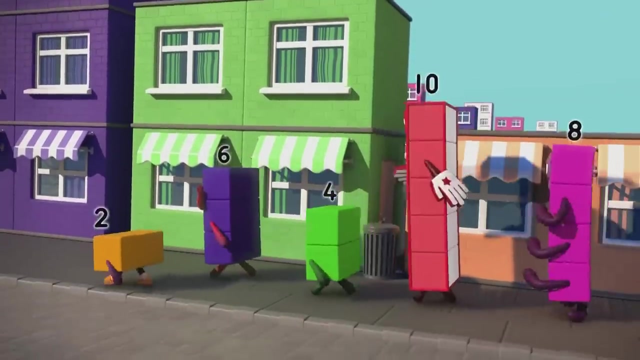 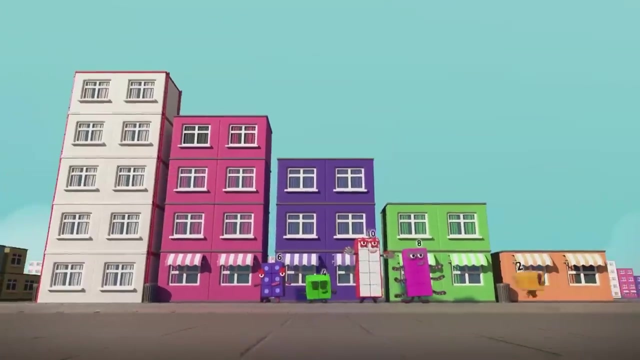 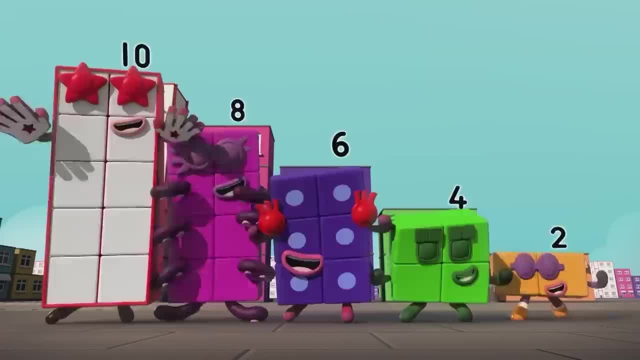 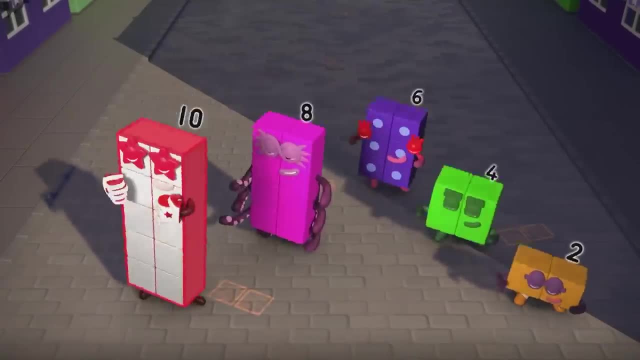 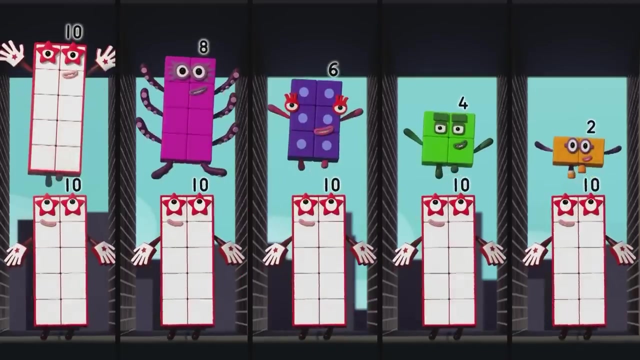 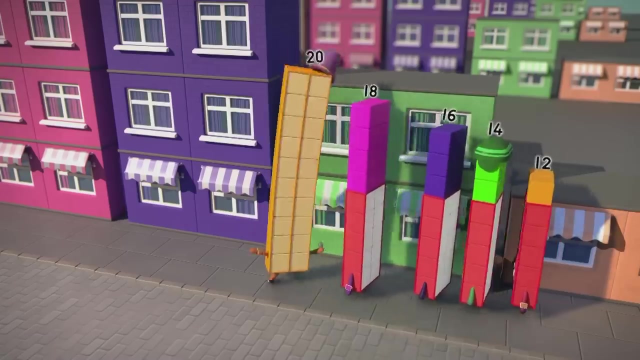 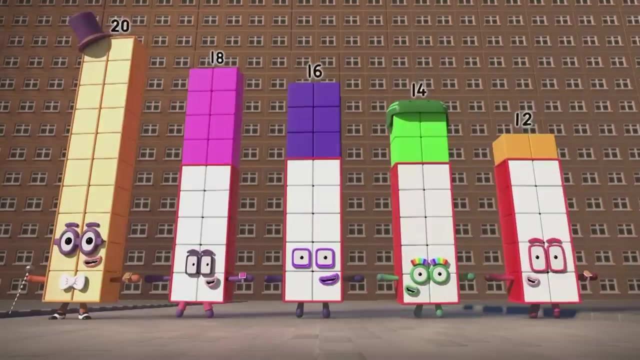 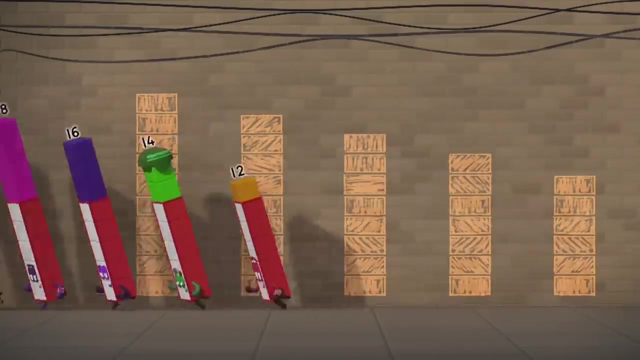 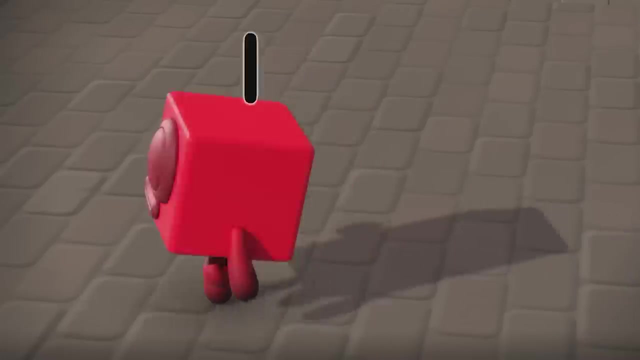 Evens Made of twos. Tens Evens Twelve, Fourteen, Sixteen, Fifteen, Sixteen, Fifteen, Eighteen, Twenty Evens Eventops. Evens Made of twos Oddblocks. 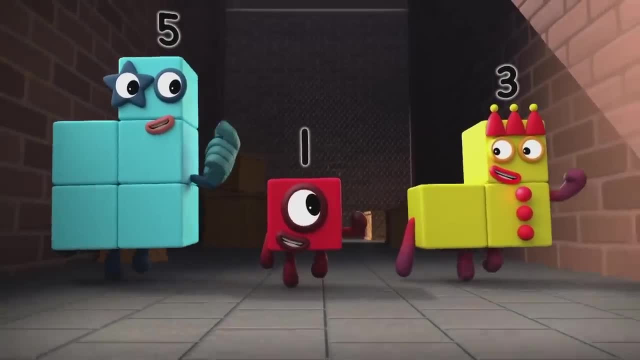 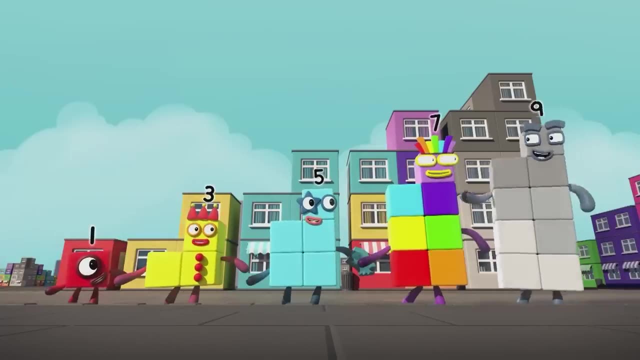 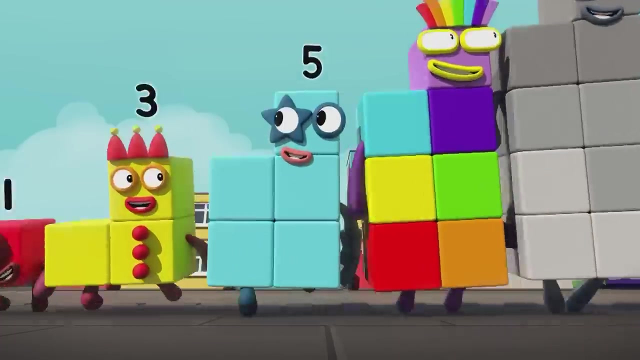 One, three, five, seven, nine, oddsss, Oddsss, Oddsss, Made of twos With a one on top Ten. Ten, Twenty, Twenty-two, Twenty-three, Twenty-four, How many Twenty-five? 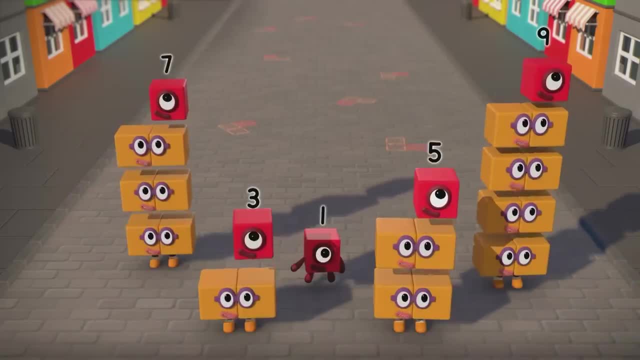 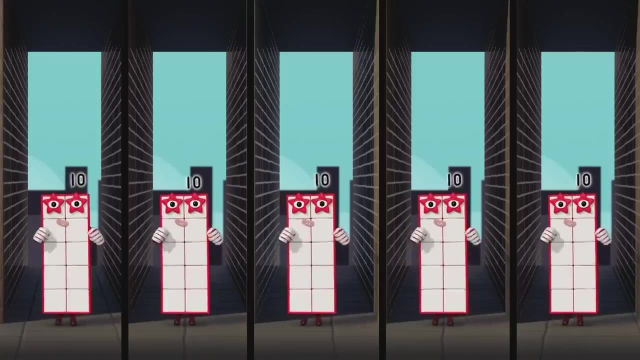 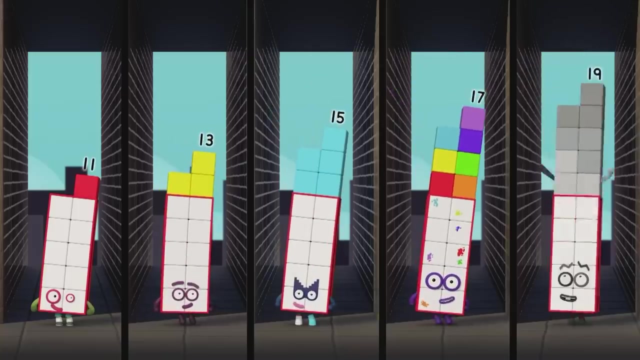 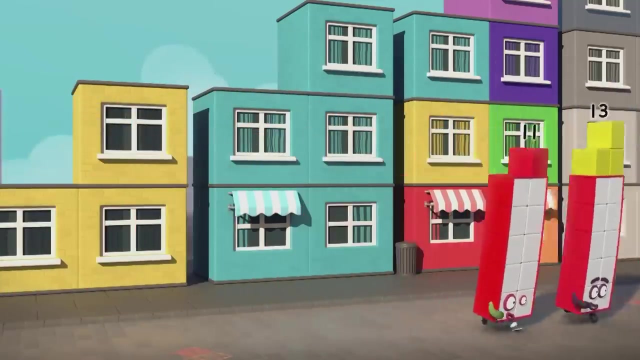 Twenty-seven, Twenty-eight, Forty, Forty, Twenty-three, Twenty-seven, Twenty-eight, Twenty-nine, Twenty-eight, Tens Odds Eleven, Thirteen, Fifteen, Seventeen, Nineteen Odds Oddblocks Odds. 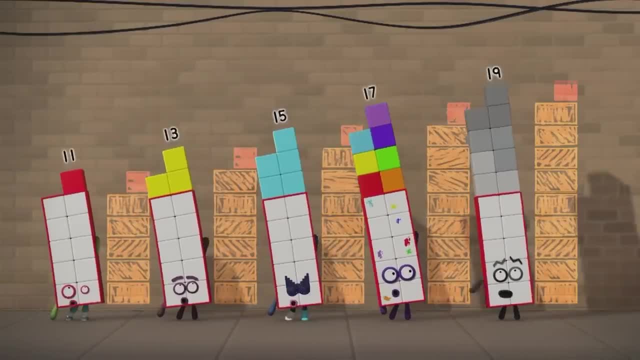 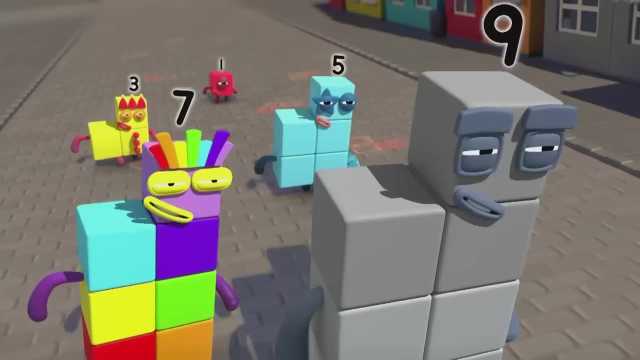 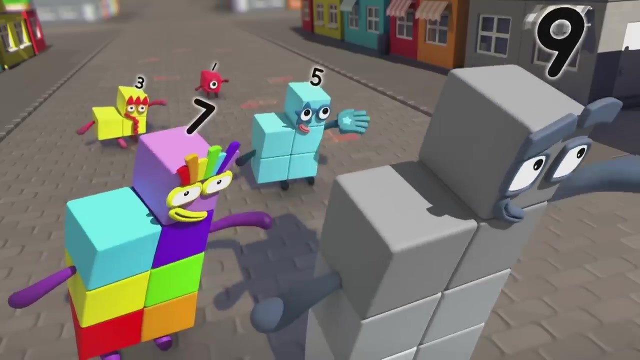 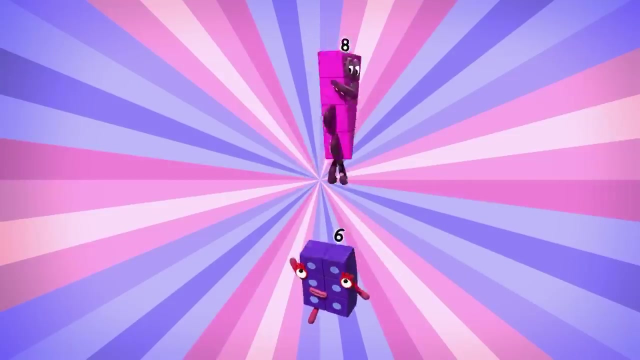 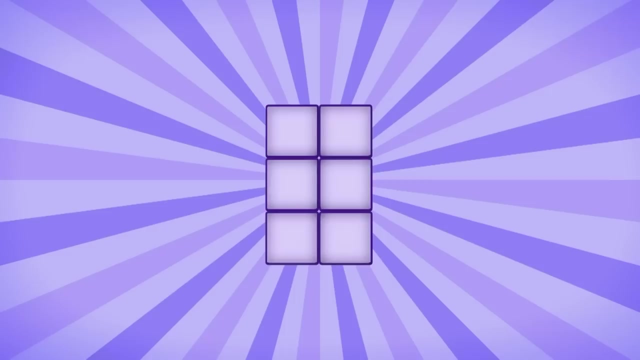 Made of twos With a one on top: Odds, Evens, Odds, Evens, Even Plus even Is even, Even. Plus even Is even, Even, Plus even Is even. Add even to even and you'll get even. 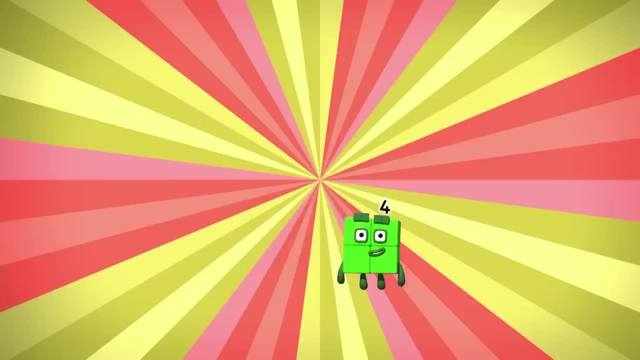 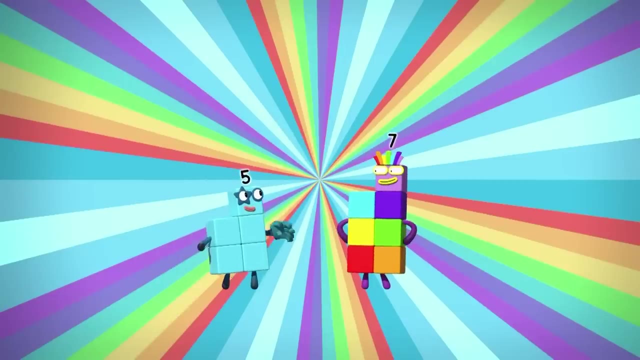 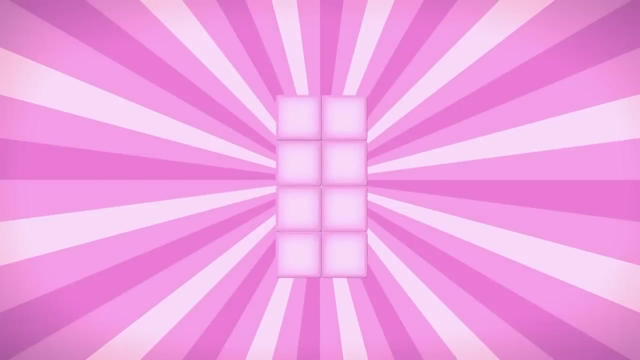 Odd Plus odd Is even. Hmm, Odd Plus odd Is even. Wow, Third time lucky. Odd Plus odd Is even: Add an odd to an odd and you'll get even. Huh, Even Plus odd. 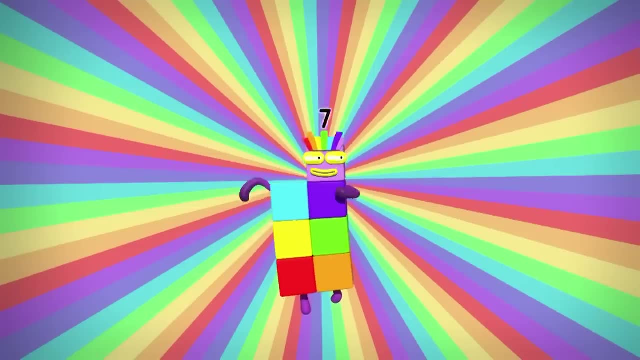 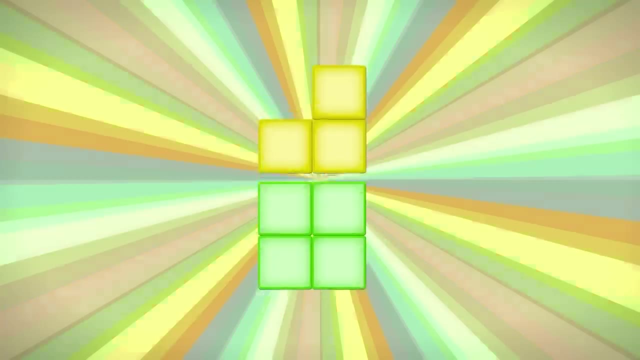 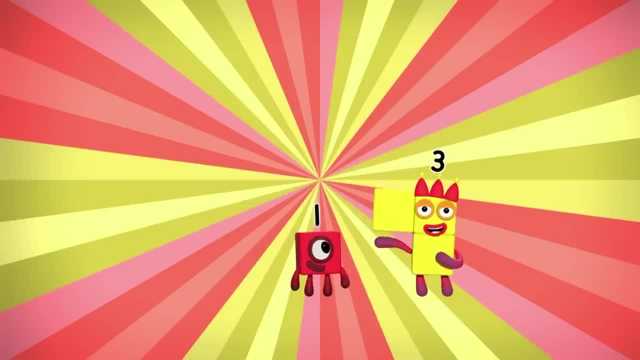 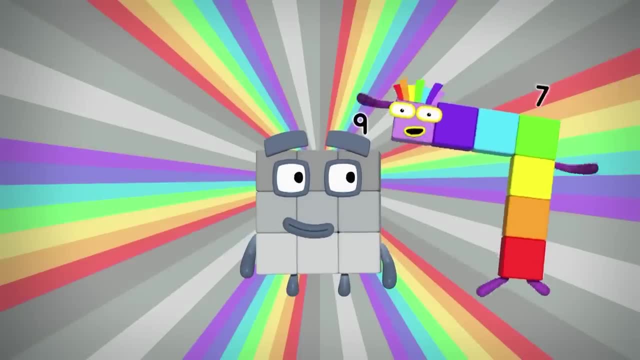 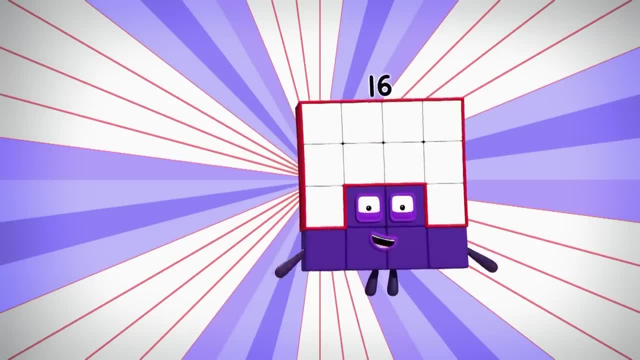 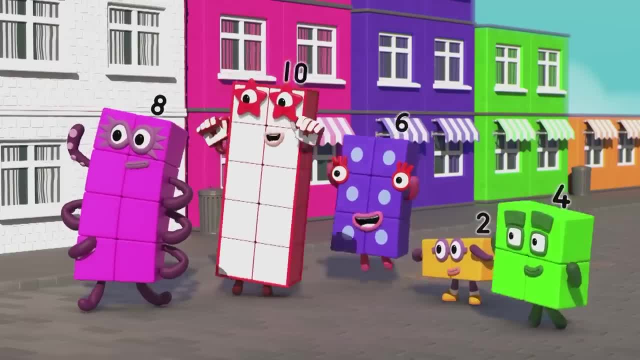 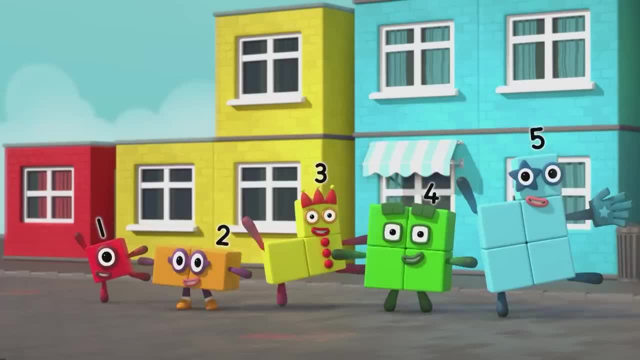 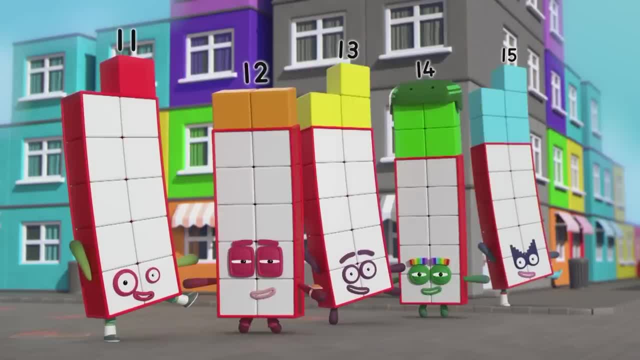 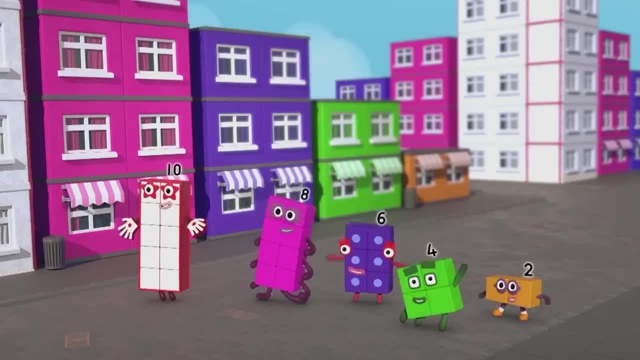 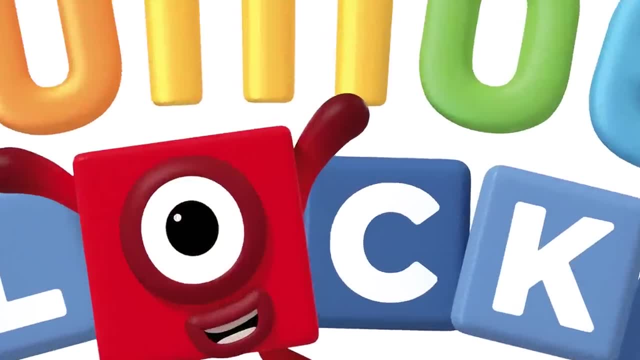 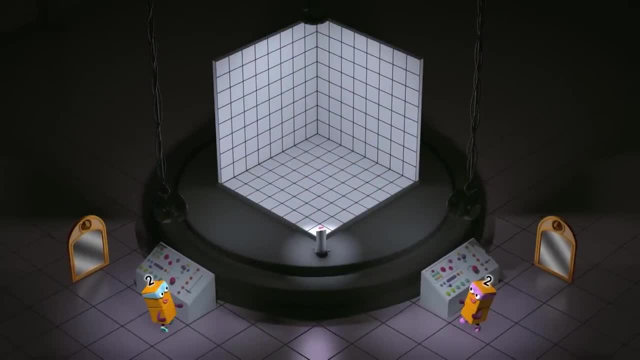 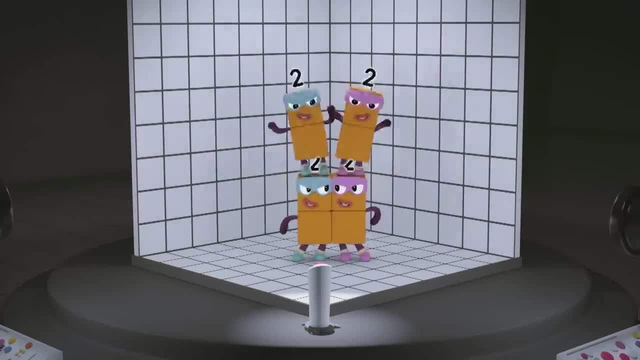 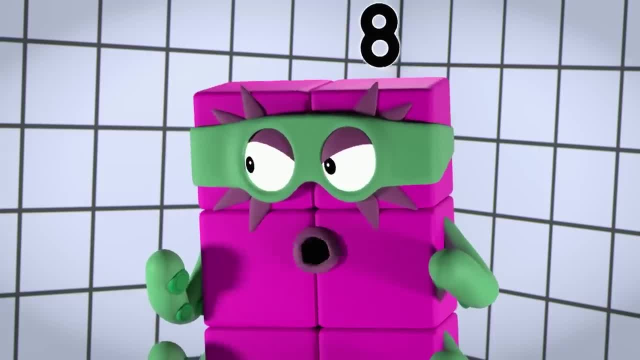 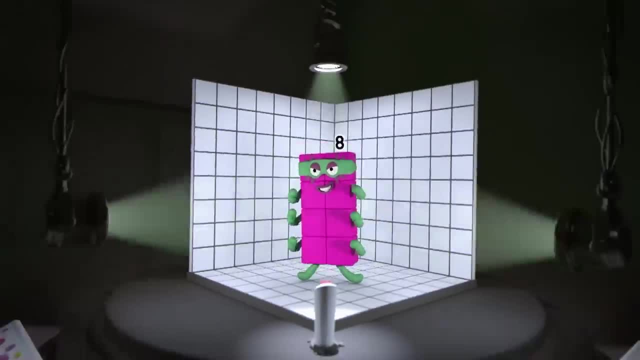 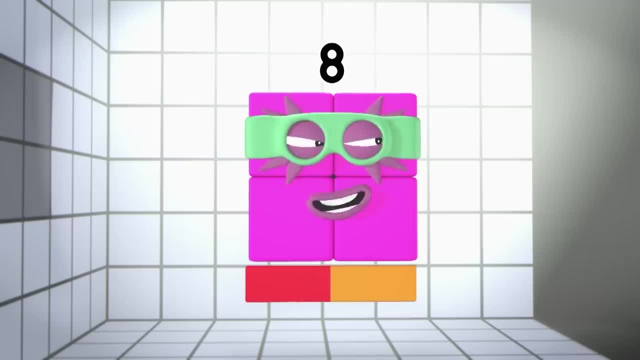 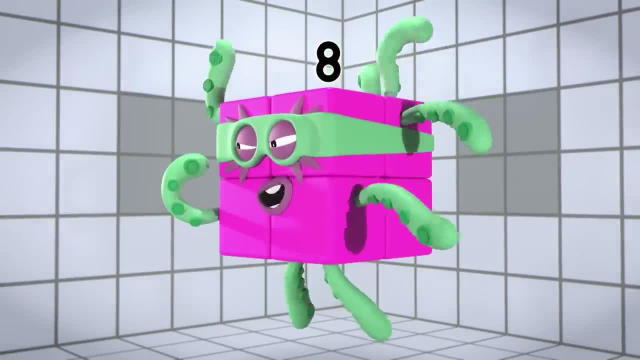 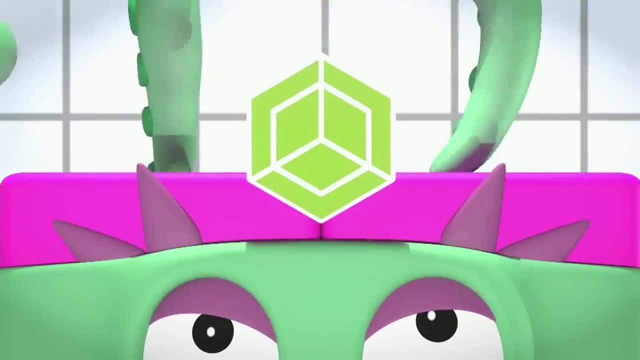 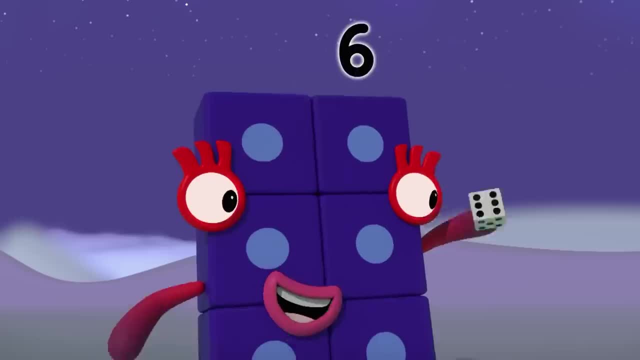 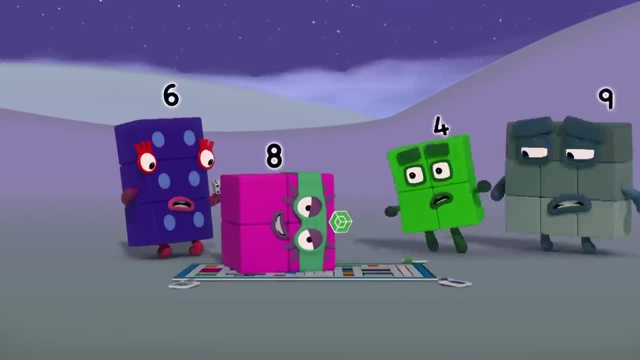 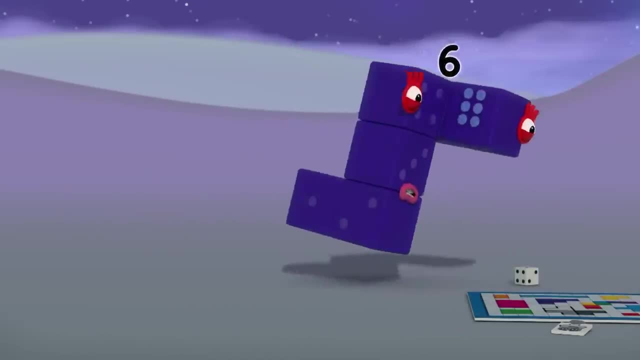 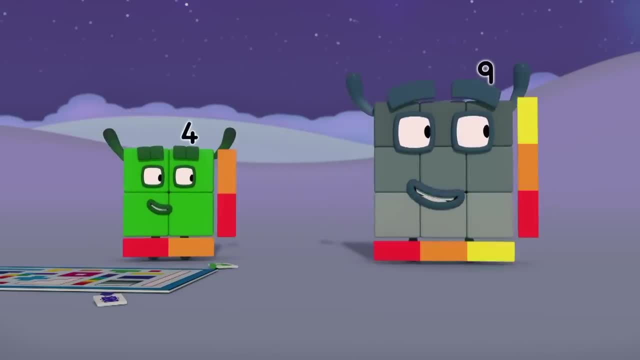 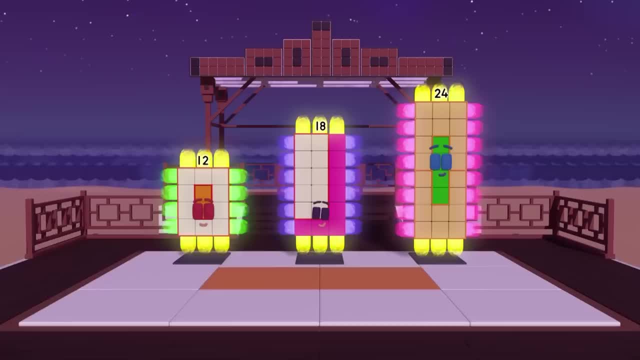 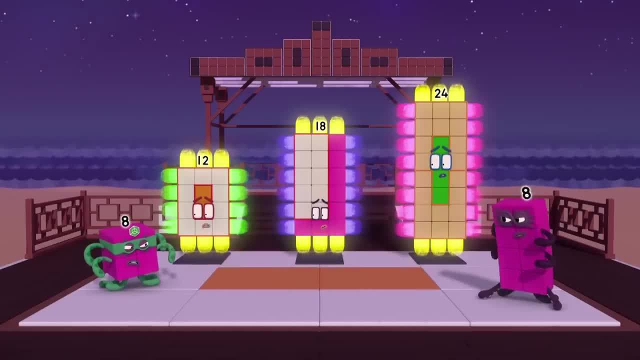 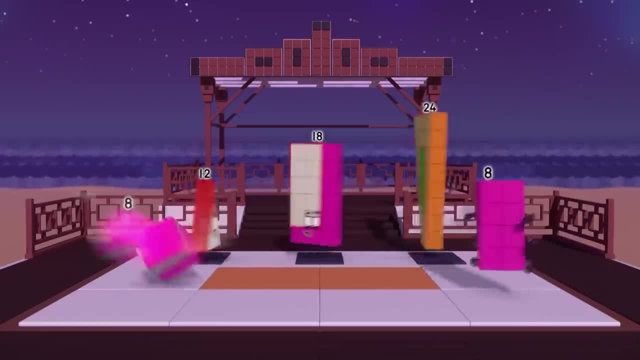 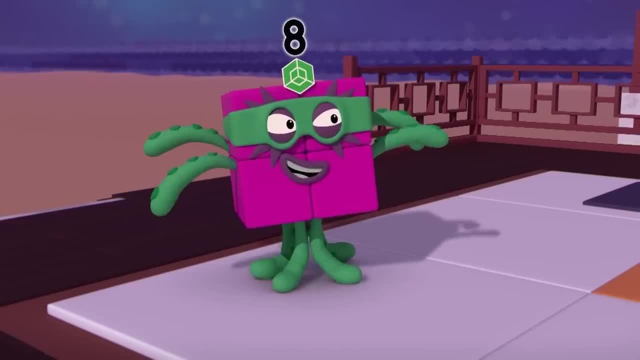 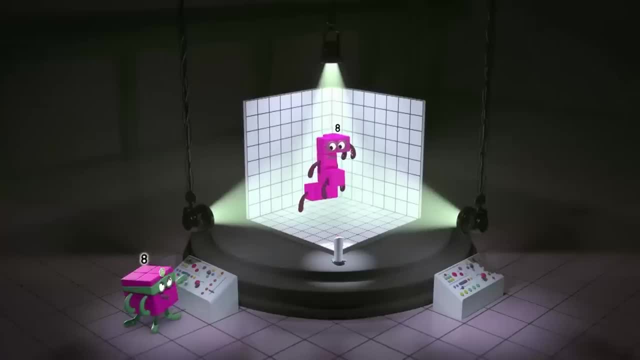 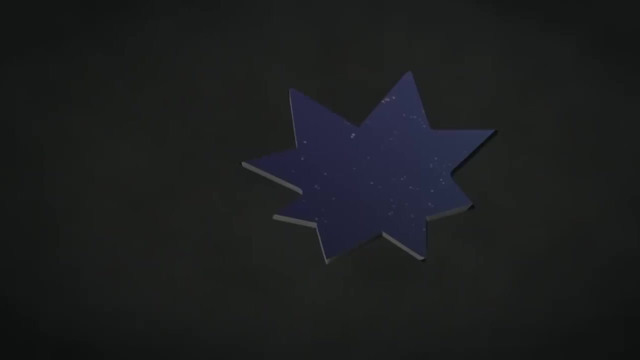 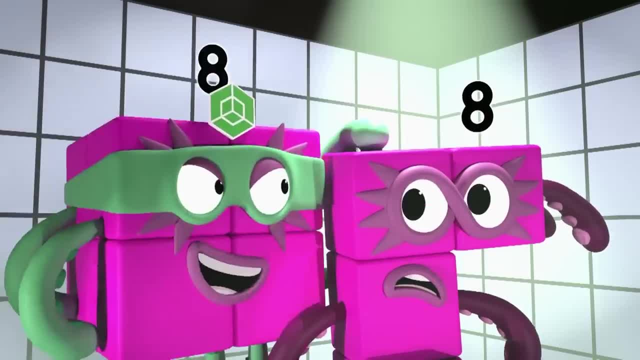 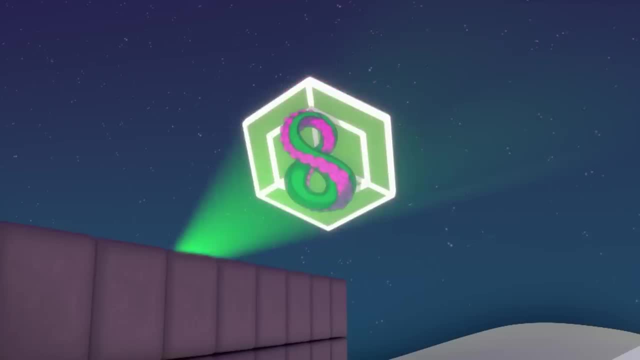 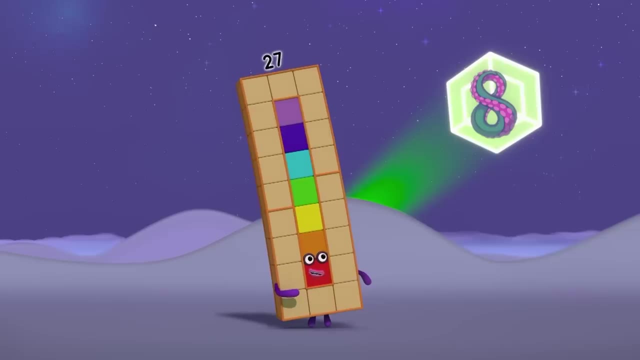 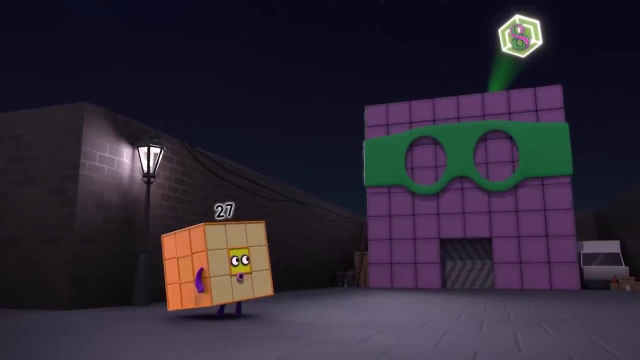 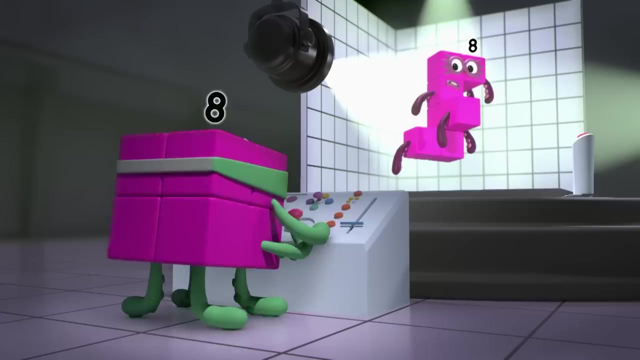 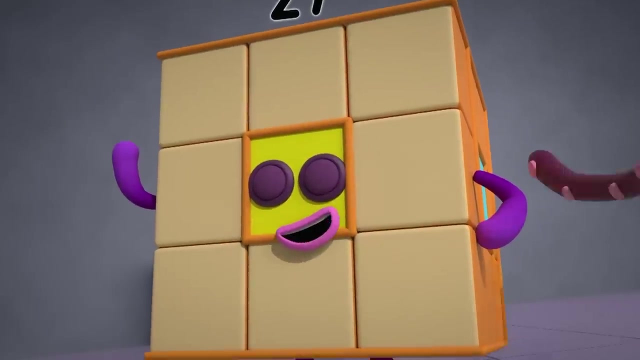 Add an odd to an even and you'll get odd. Add an odd to an even and you'll get odd. Add the odd to an even and you'll get odd. Add an odd to an even and you'll get odd. Add an odd to an even and you'll get odd. 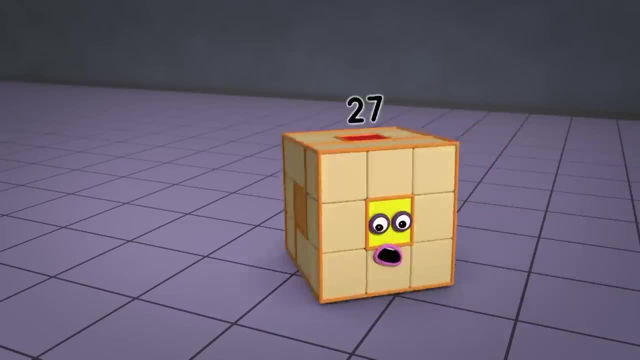 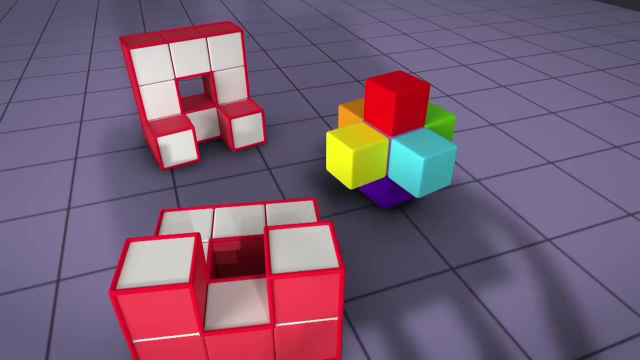 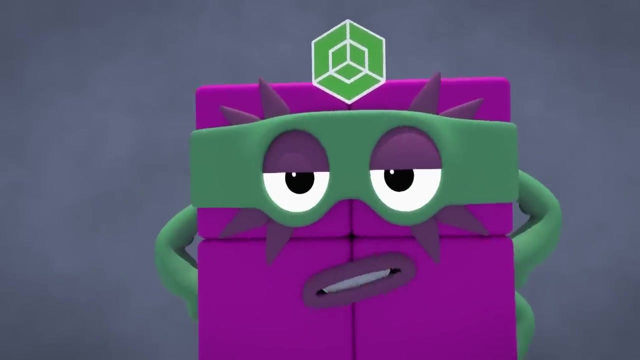 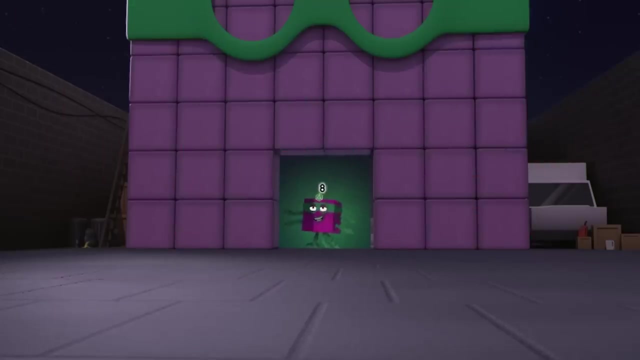 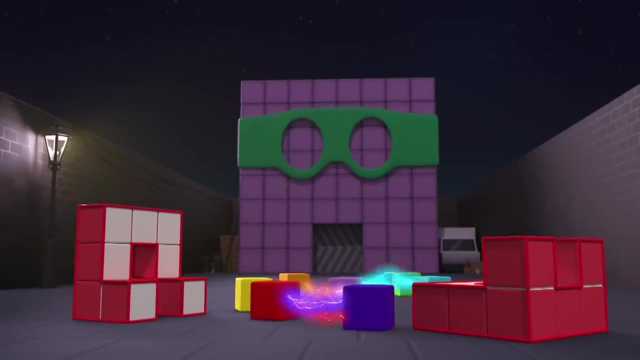 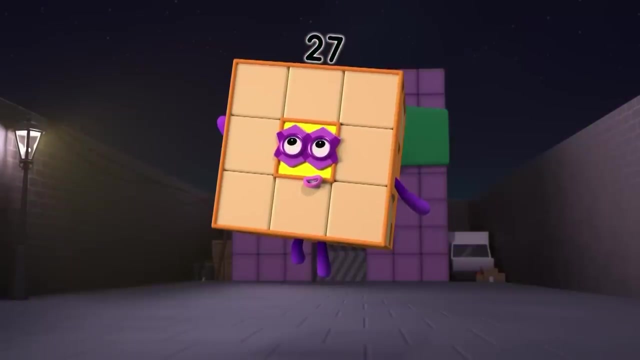 Whoa, Ah, Bit of a mess. I'm the only cube allowed around here. The rest of you will be wonky shapes forever. Now let's have no more distractions. As I was saying, I am 27 and I am a super-cube. 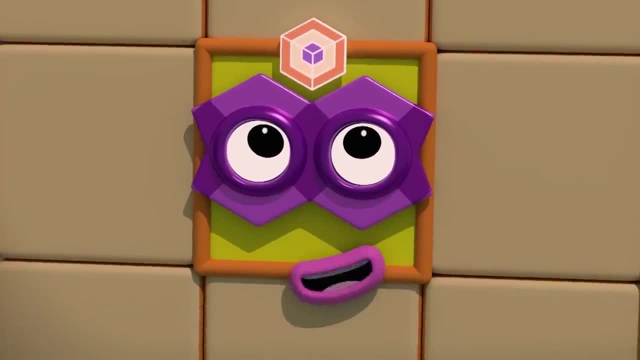 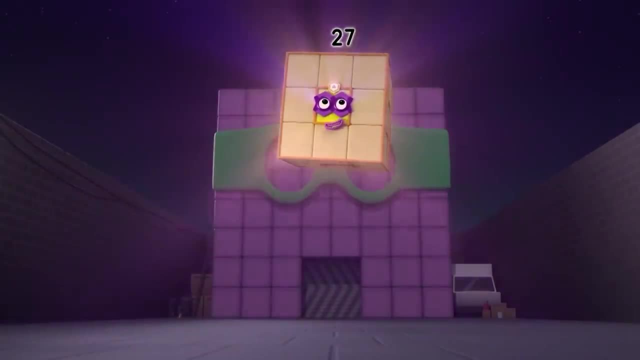 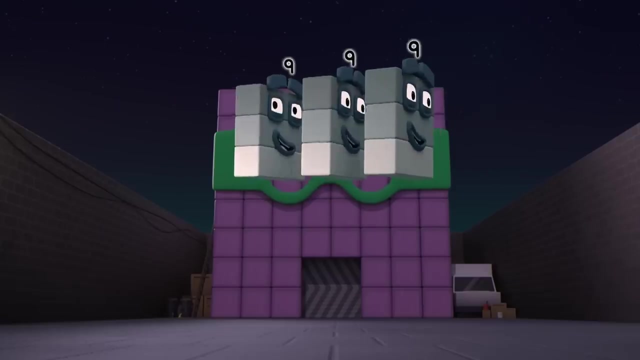 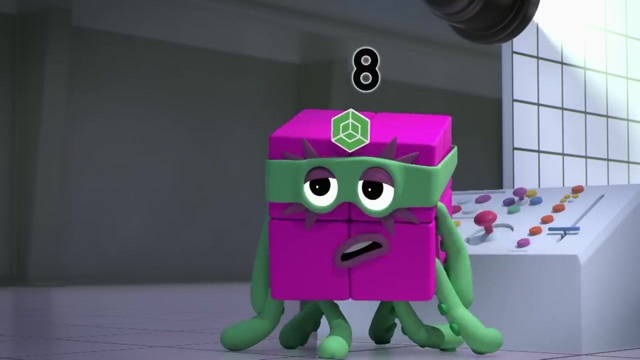 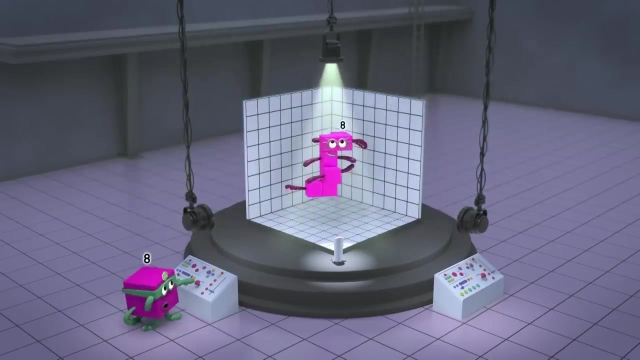 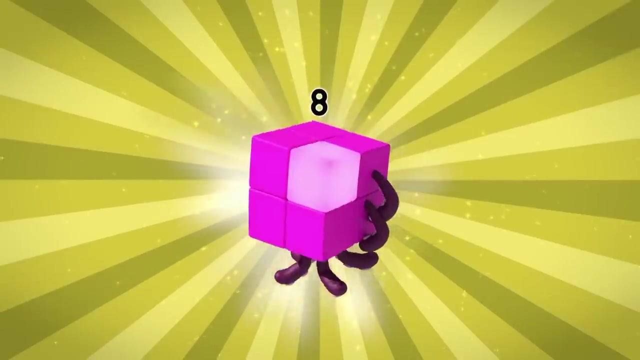 Three by three by three, By the power of three Dimensions, The three nines Super-sneeze, Ah-choo Ah. Octo-cube One, two, three, four, five, six, seven, eight Octo-cube. 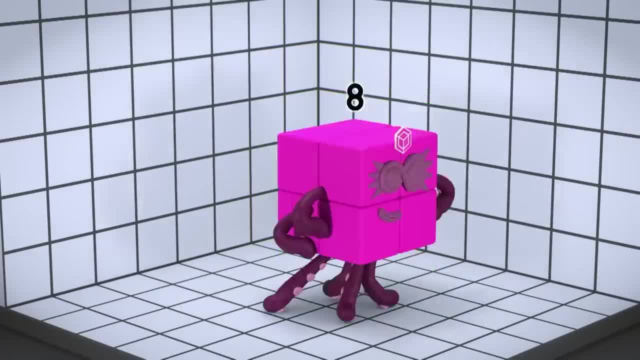 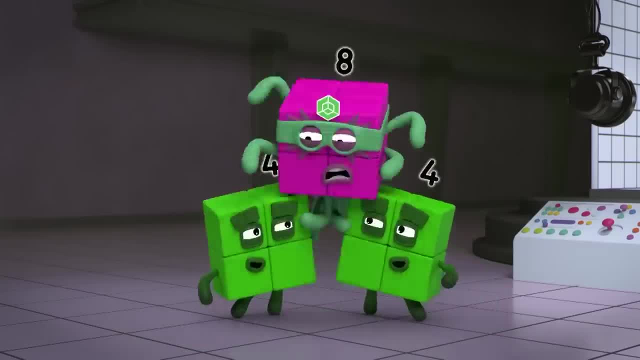 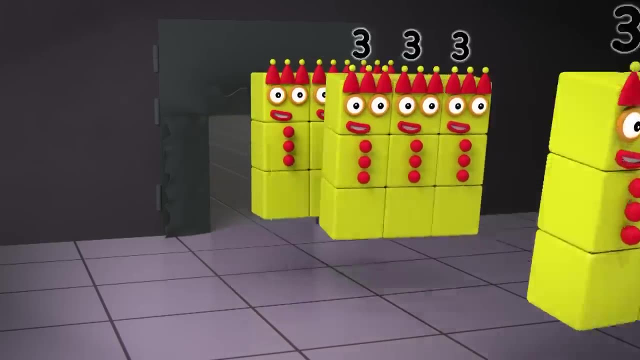 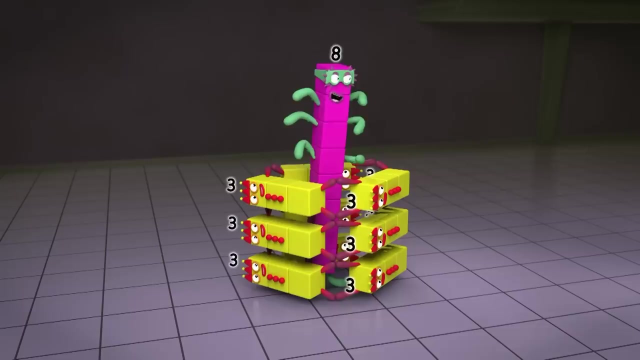 By the power of three dimensions, The fantabulous fours, Nice is stronger than naughty. By the power of three dimensions, The three, three, threes. Smile please. Ah-hah, The Dimensionator will make me a super-powerful cube again. 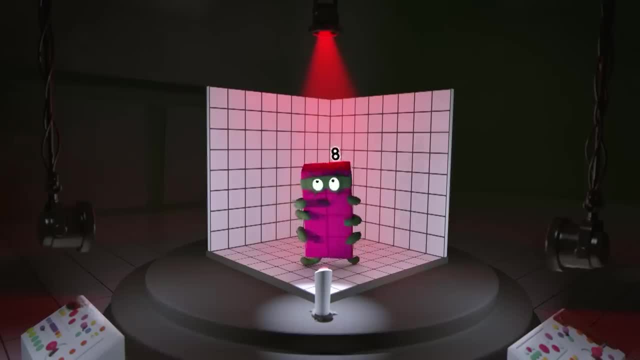 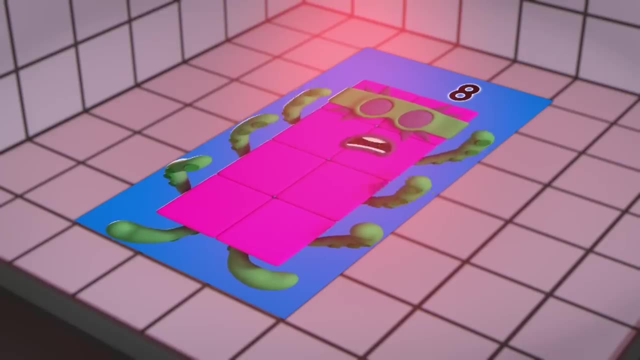 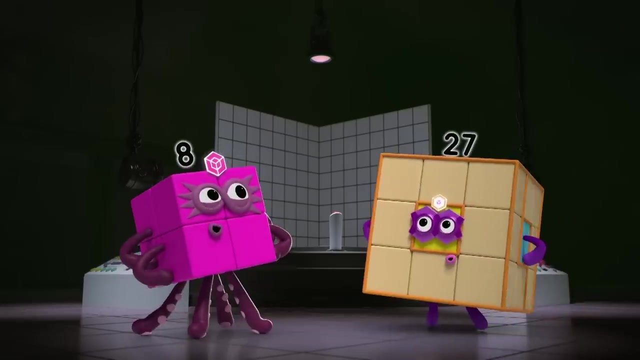 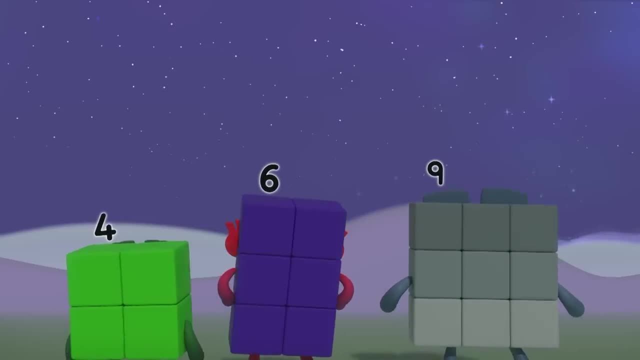 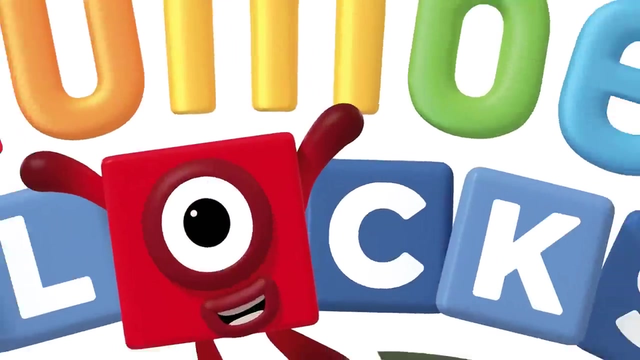 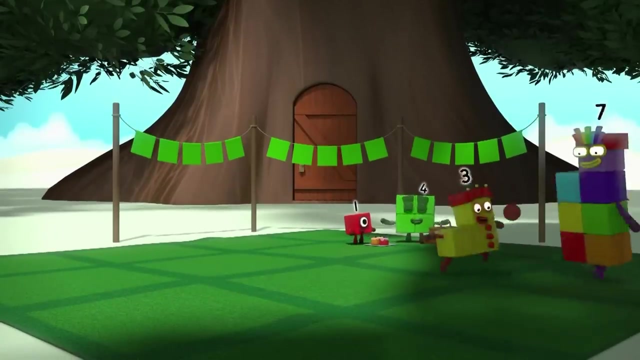 Woo-hoo, I'll get you next time. Octoblock By the power of three dimensions. Hoo-hoo, If there's one thing better than a picnic, it's a square-club picnic. Ha-ha-ha-ha-ha-ha-ha. 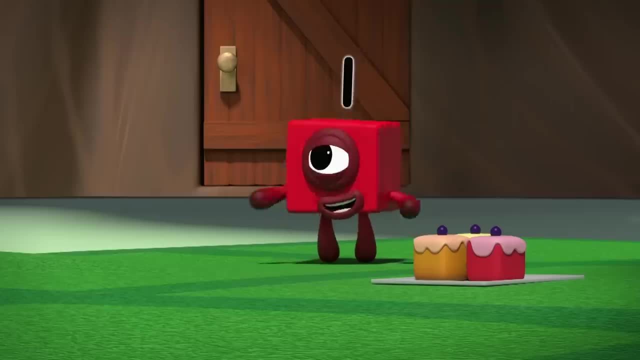 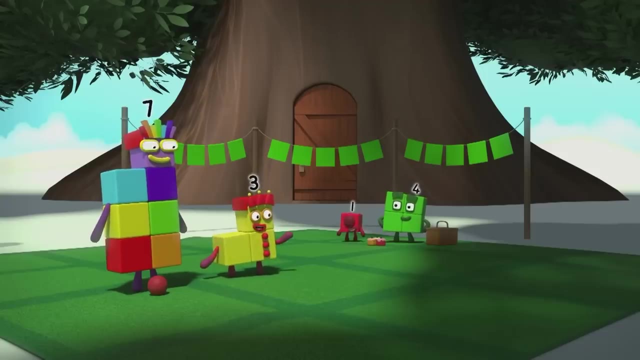 Hey one, See you at the Outlooks picnic. I'll be there soon. Club Picnic Day is a busy day for me. Tell me about it. We've both got the Step Squad's picnic later. You too. Twenty-One 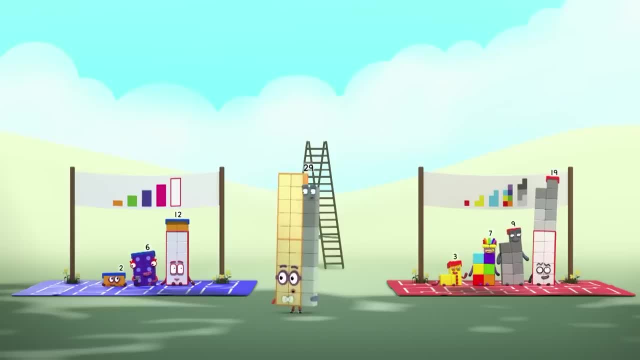 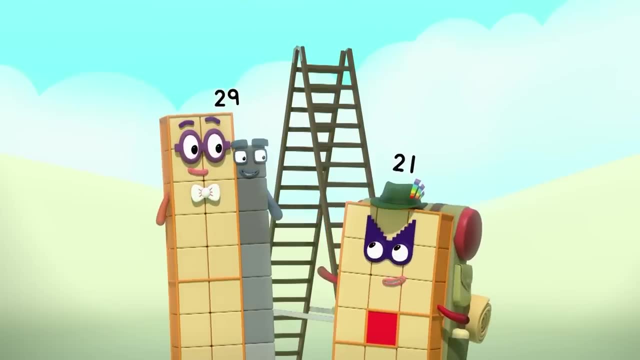 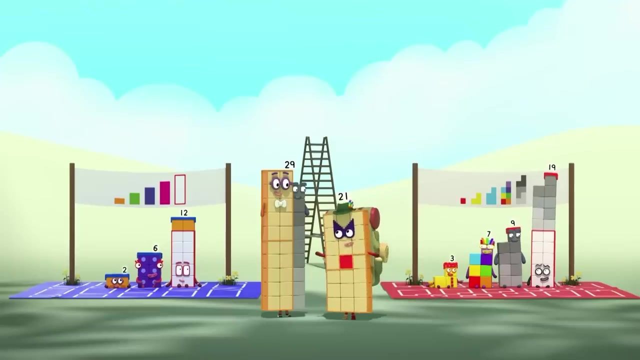 See you there. three Wow. I've never seen so many clubs. It's Club Picnic Day 29! Wow. Sniffing your clubs helps you discover what you have in common with other number blocks. For example, do you fit in with the odd blocks or the even tops? 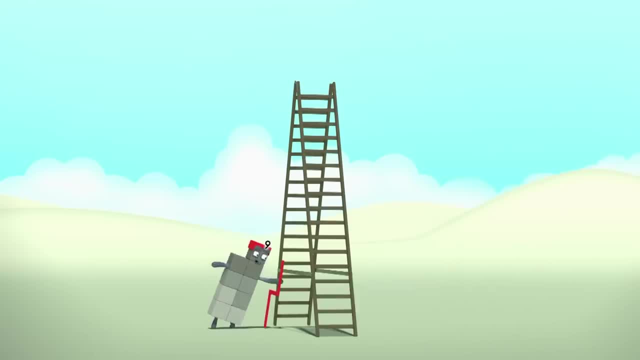 Come and find out. The rule is: when you stand two blocks wide, if you've got an odd block on top, you're in the odd blocks. Ha-ha-ha, I did it. I fit the rule. I fit in with the odd blocks. 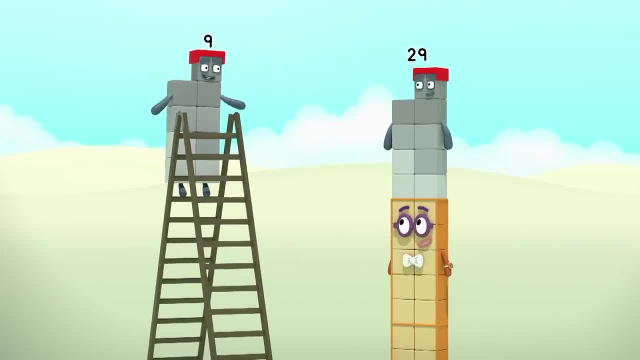 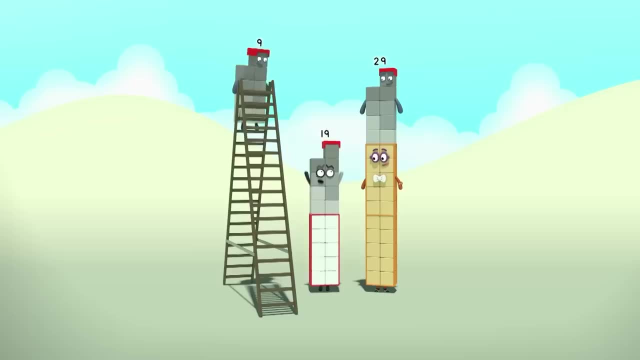 I thought you might. You end in a nine, you see, And any number that ends in a nine is odd, like me And me. Welcome to the Club 29!. I like the helmet. It's nice having something to show on a member. 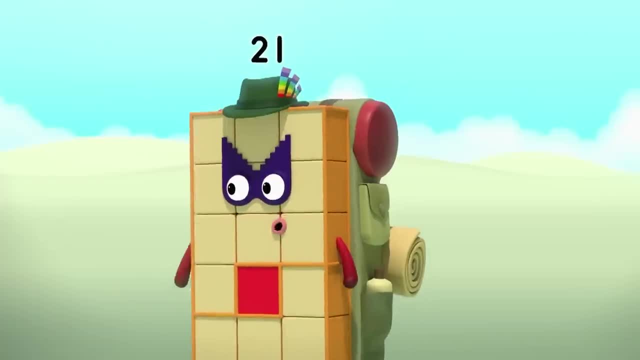 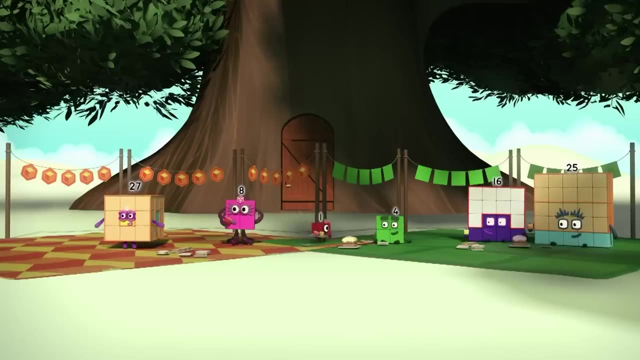 Are there any more clubs I can join? Let's go and explore. Everyone knows Square Club. Oh, hello there. I thought it might be fun to start up a cube club And since I'm in both clubs, this saves me some running about. 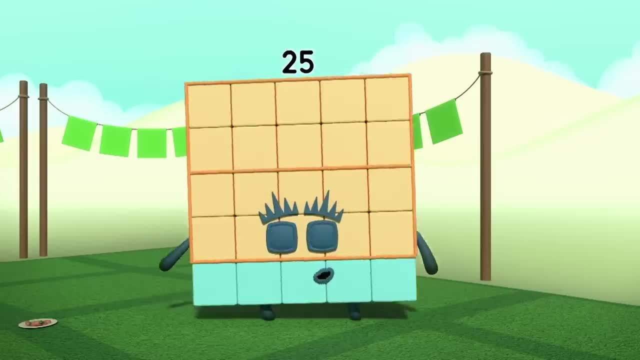 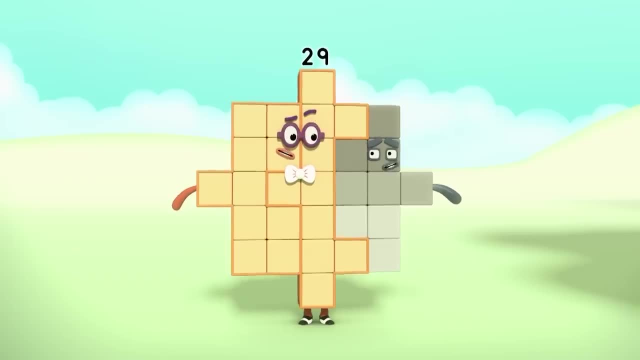 Blockcake-ate, Blockcake-ate, Ha-ha. You can join Square Club if you can make a square and be as tall as you are wide. Hmm, don't think so. To be in Cube Club, you need to be able to make a cube. 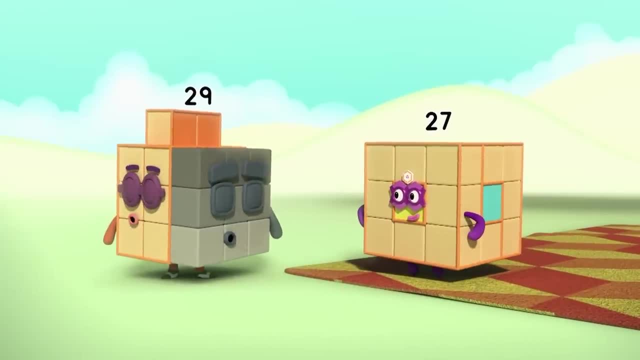 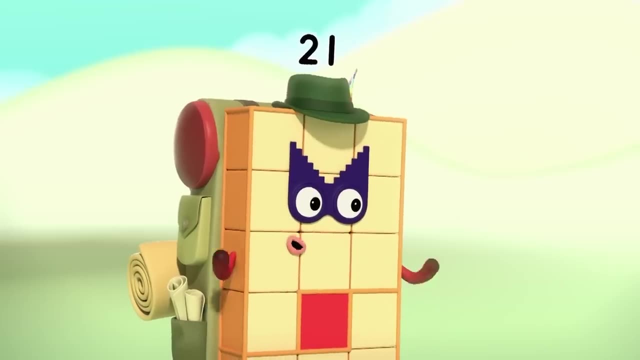 Like this: Hmm, no, But you said this was a new club. Does that mean that anyone can make up a new club, I suppose. so You just need a rule about who gets to be in it, Like Nine Enders. 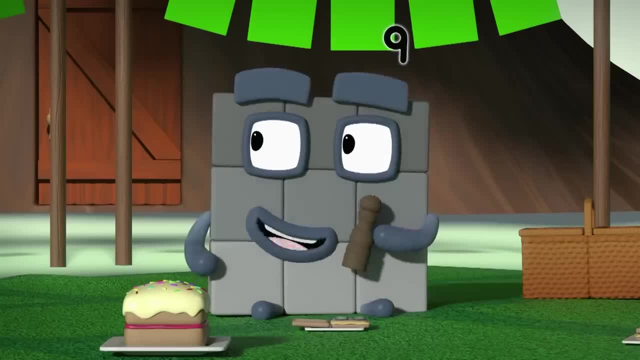 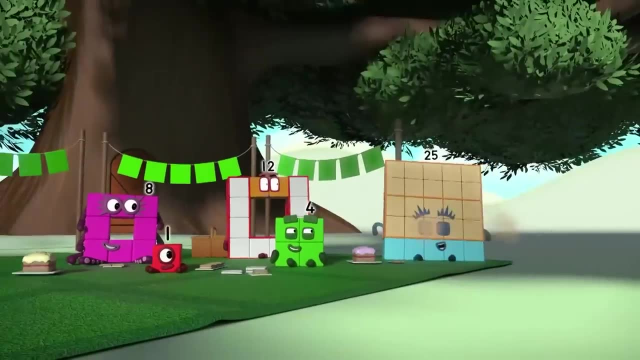 The club for numbers who end in a nine. I like the sound of a A-choo Ha-ha, A-a-choo, A-a-choo And me-choo Ha-ha. Squares with holes in. 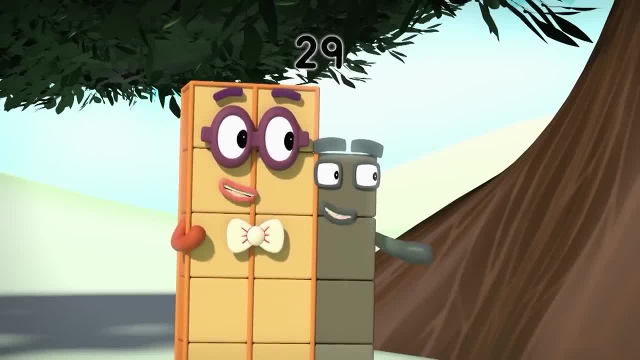 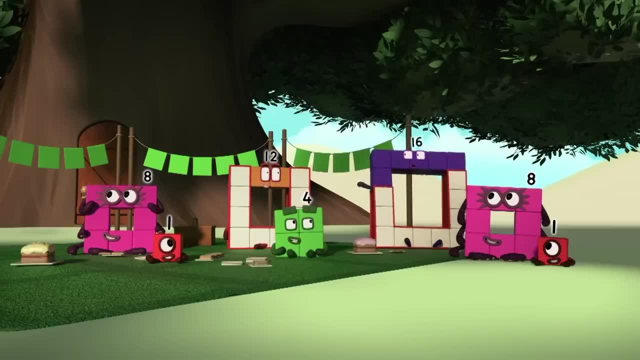 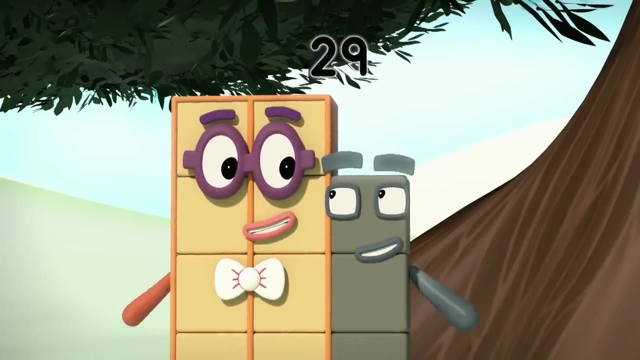 Ooh, how about a Squares with Holes in Club For eight and twelve and sixteen and anyone else who can make a square with a hole in? Why not? Anything to do with squares Sounds fun to me. There are so many new clubs I could come up with. 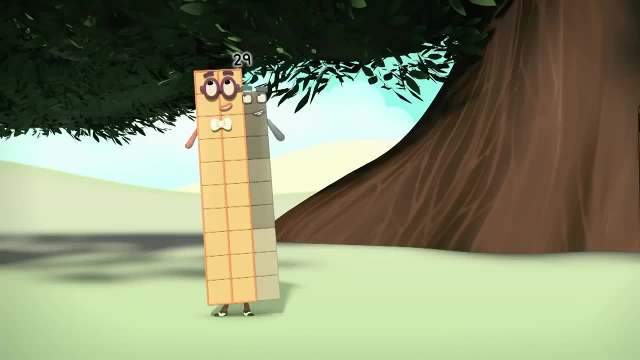 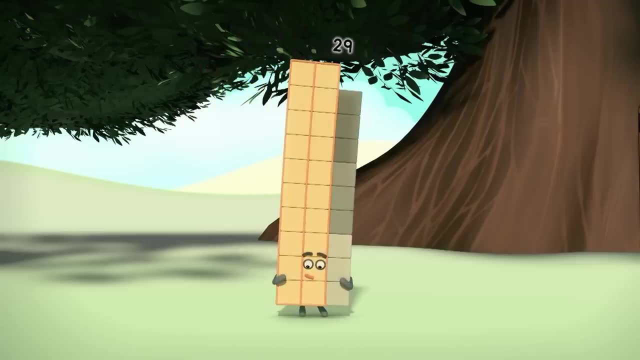 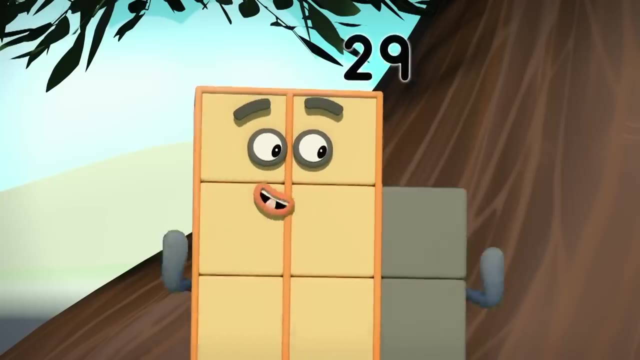 I've figured myself out. I'm Twenty-Nine And I love clubs, Being in them and making up new ones. Like Square with a Hole in Club. You need something to show you're all members. Like badges- Club badges There. 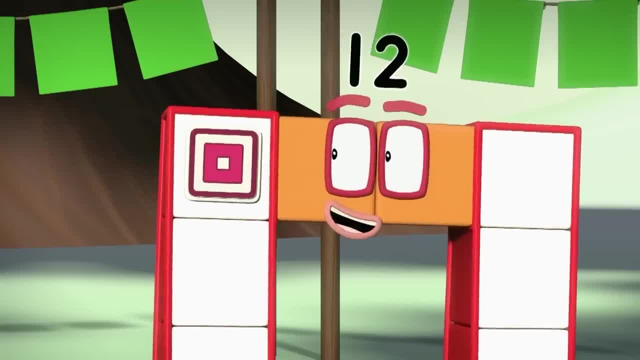 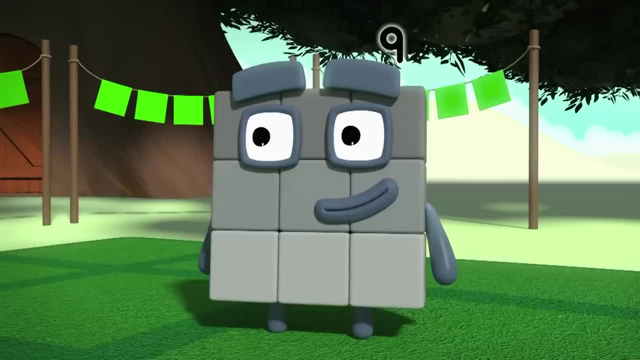 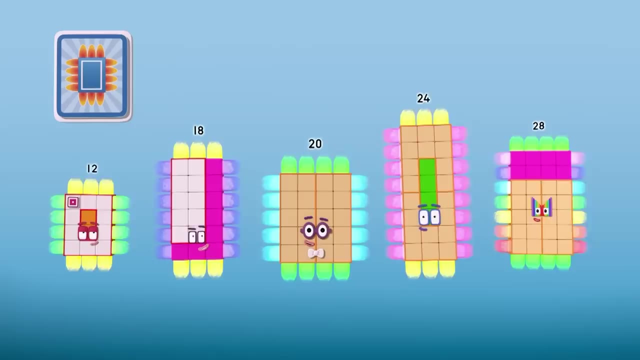 Square with a hole, Ha-ha, Ha. Oh, And how about square badges for Square Club? Ho-ho, Ooh, thank you Twenty-Nine. Hey, I'm only just getting started. Super Rectangles Club- Hooray. 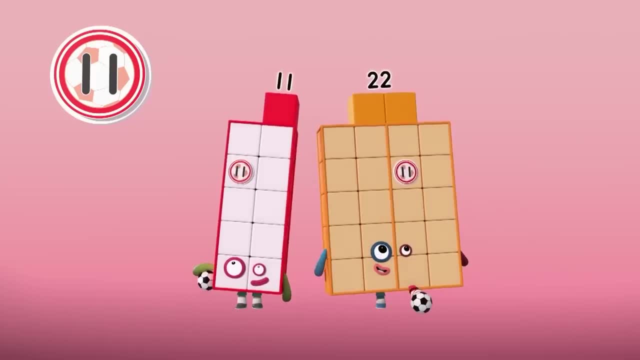 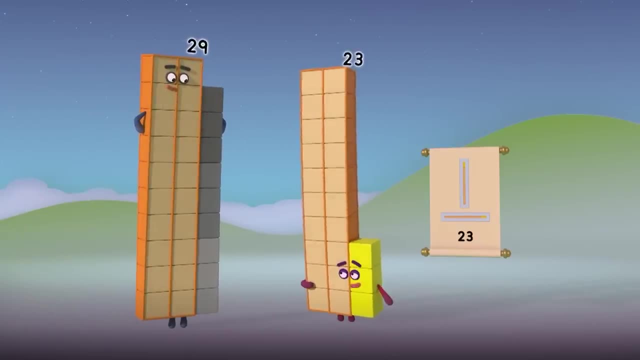 Step Squads: Hooray League of Elevens: Yay, Um, can you make lots of rectangles? Quite the opposite. I'm a not very rectangular number who can only make prime positions and no others. That's a bit of a mouthful. 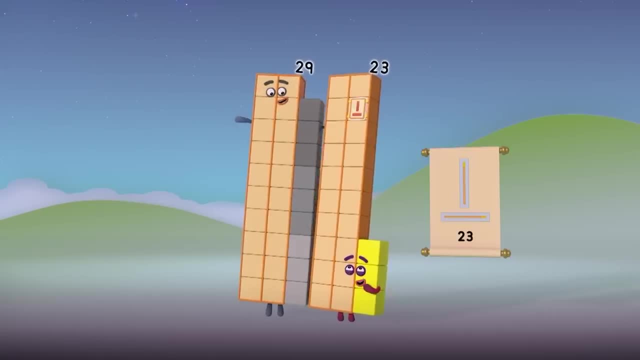 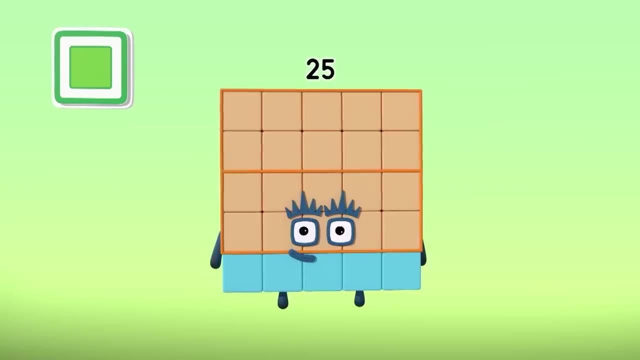 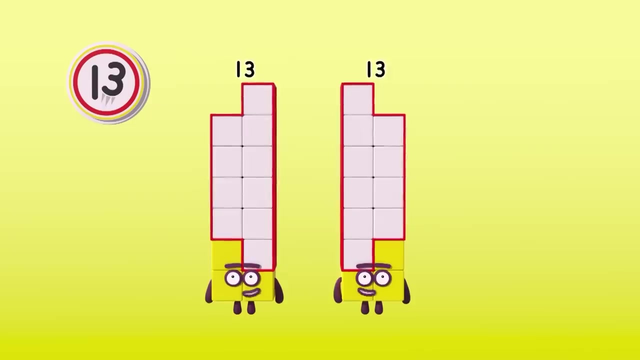 How about Prime Club, Whoa, Whereas you're even more rectangular. Super-duper. Rectangle Club for you, Oh. Square Club, Oh, You're in the Undercover. Thirteens Club Twenty-Six, Ooh, Double Thirteen. 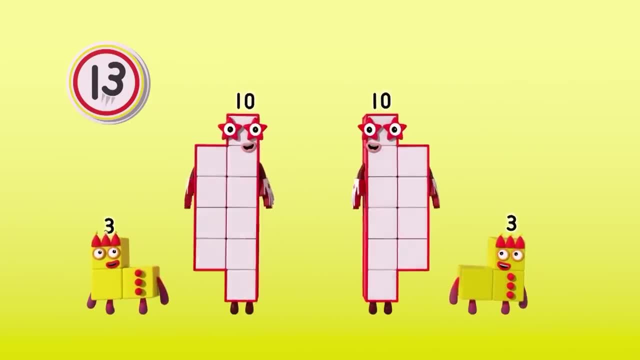 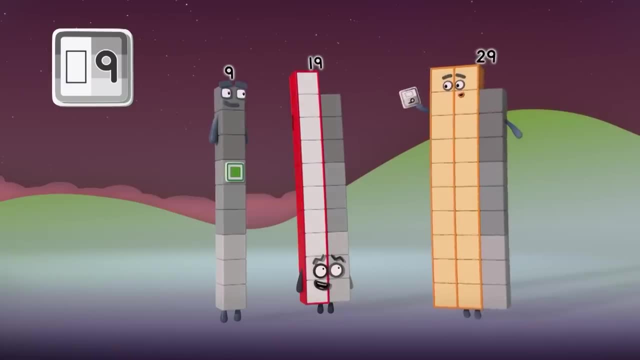 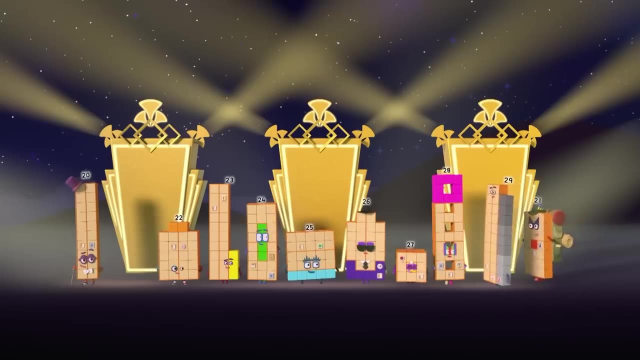 Oops, Oh, Um Falling Apart Club. Cube Club, Oh. Rainbow Sevens, Yay, And my new club, the Nine Enders. I've got one more club for you, The Roaring Twenties All together now. 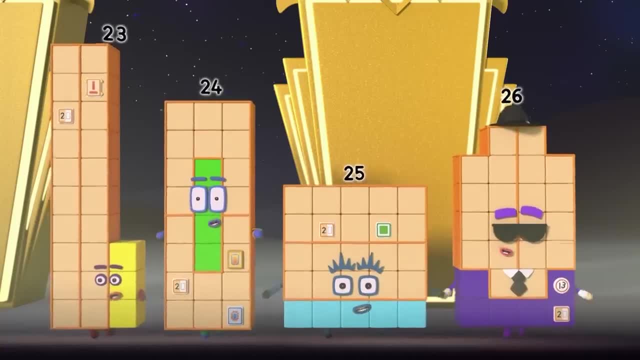 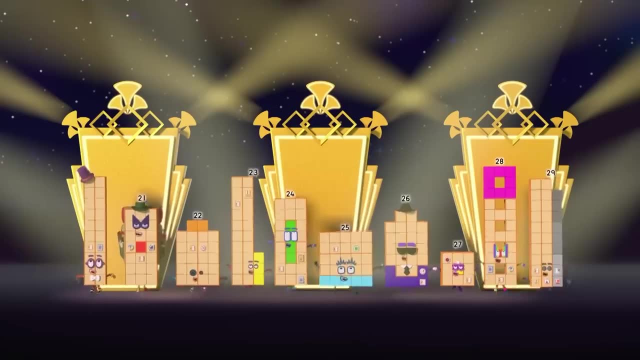 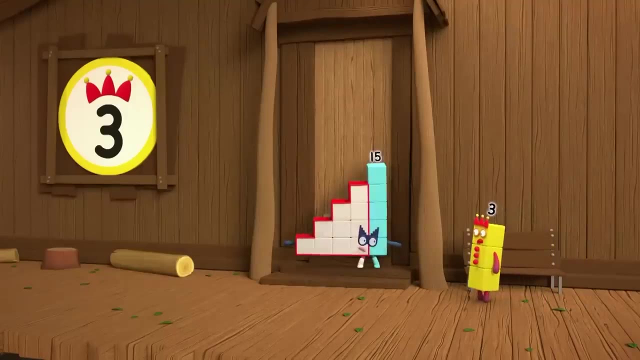 Twenties, Twenties, We're the Roaring Twenties. Get in line, feeling fine. Twenty up to twenty-nine. Oh, Three, You're early. I mean you can't come in, But it's the Three. Club meeting, Yes, but 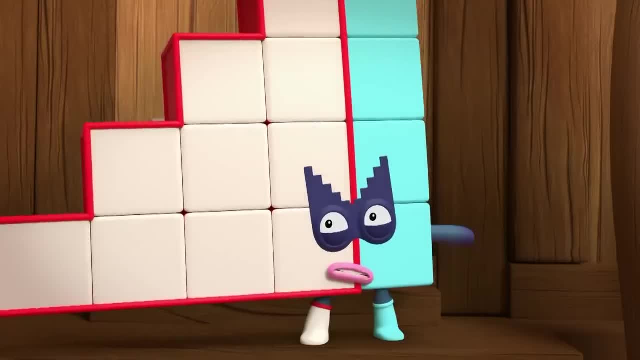 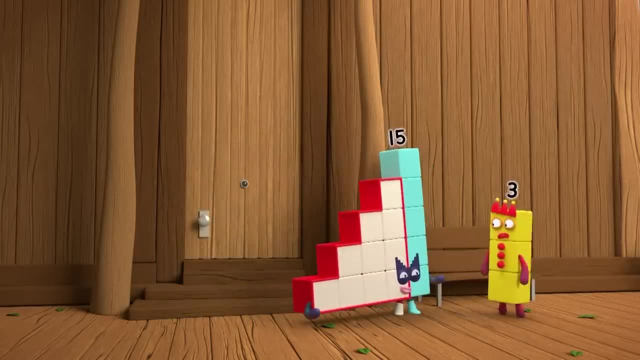 It's such a lovely day, Why don't you Get bird-watching first? I love bird-watching, Great See you later. Oh Oops, Forgot my trinoculars. Oh Oops, Forgot my trinoculars. 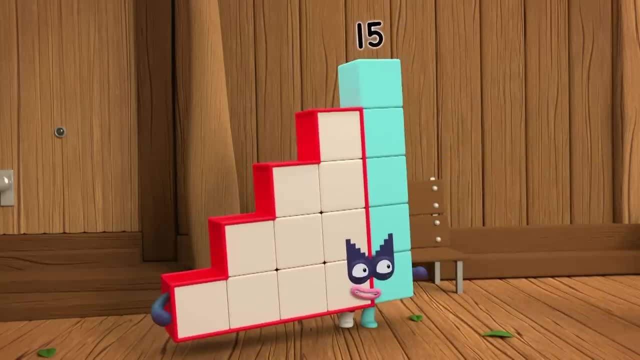 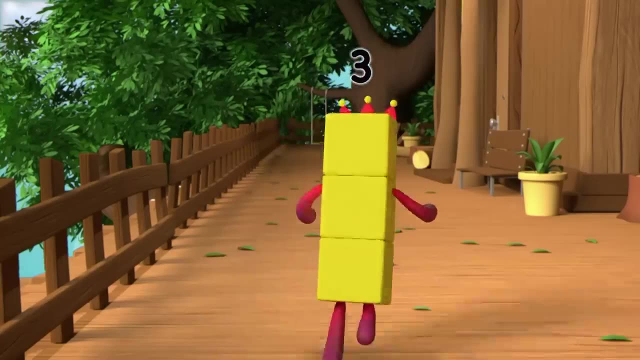 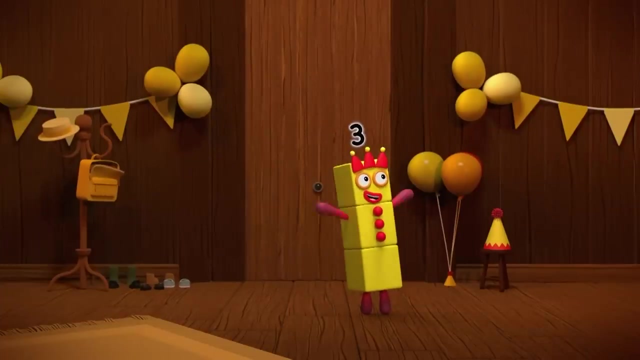 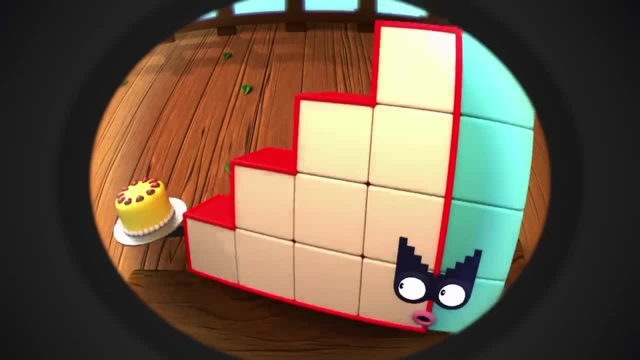 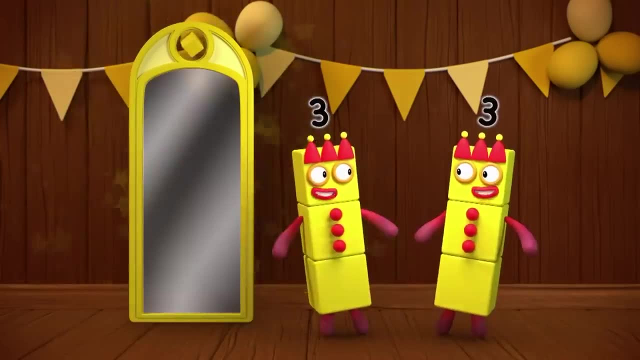 Oh, Oh, 15!. She told me not to come in. Better not let her see me. Ha, Two, threes are Two, threes are Six. Thank you Six. You're early. Yup, Just me. Definitely not three. 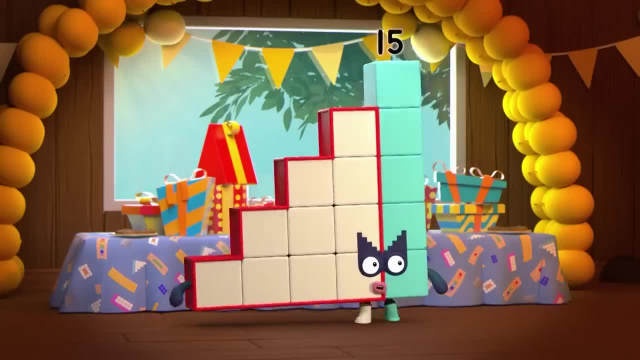 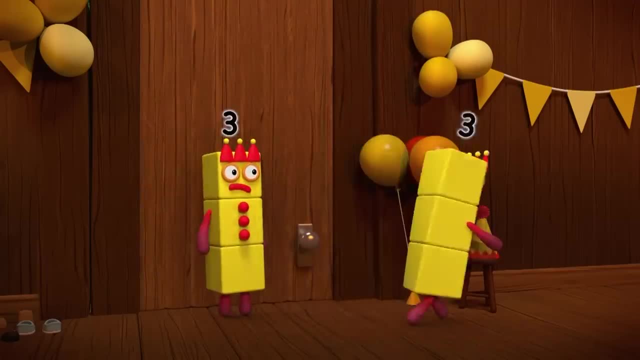 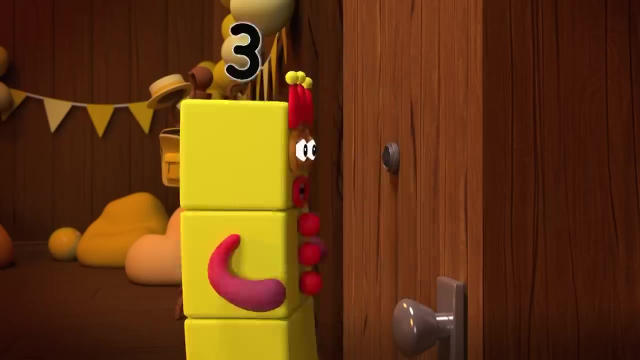 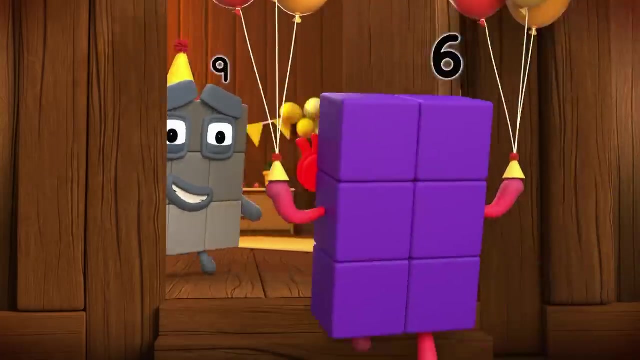 Hush, Hush. Remember, whatever you do, Don't let three in A party. how exciting, But we're not supposed to be here. Let's go before It's six. Quick hide Three. threes are Nine. Hello, nine. Why this looks fine. 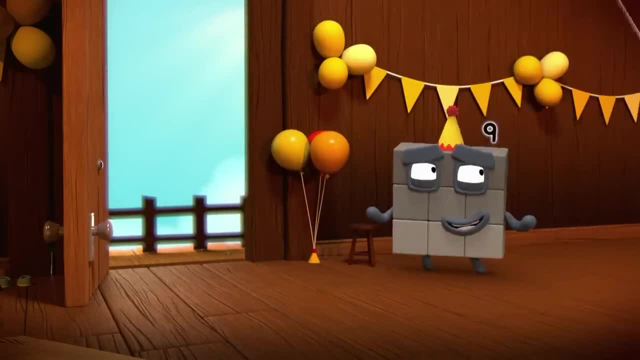 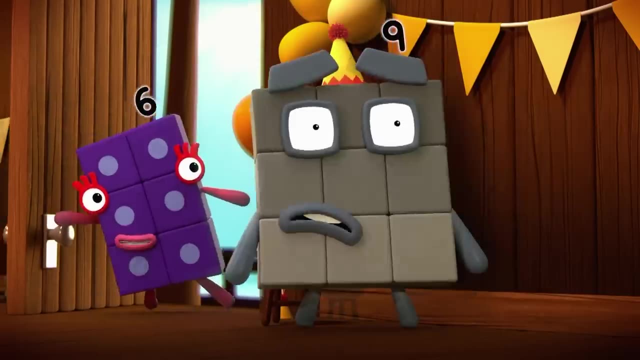 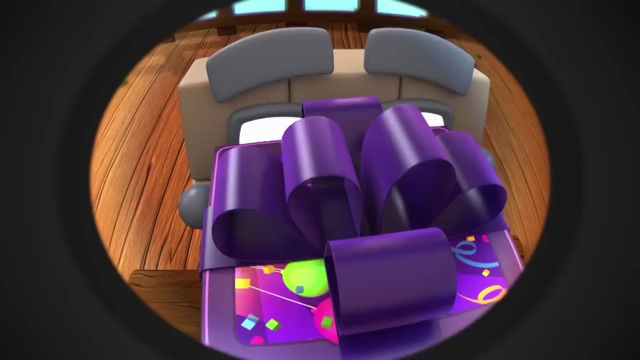 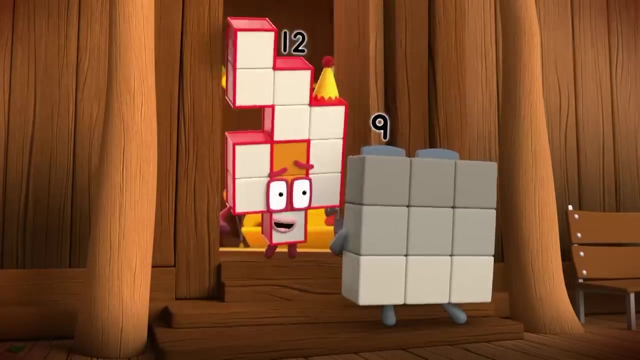 You haven't seen three, have you? Just me, myself and I. Good moustache, but I'll be back in a flash. Nice hat, That was close, Let's go before It's real. nine Hide Four. threes are Twelve. Funny, I thought I heard three. 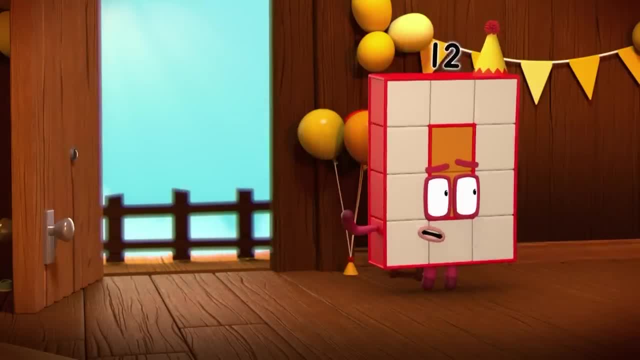 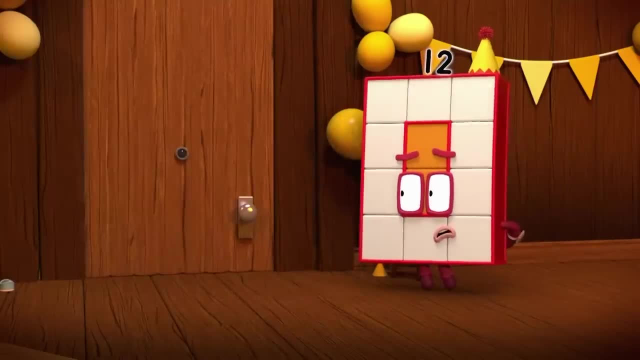 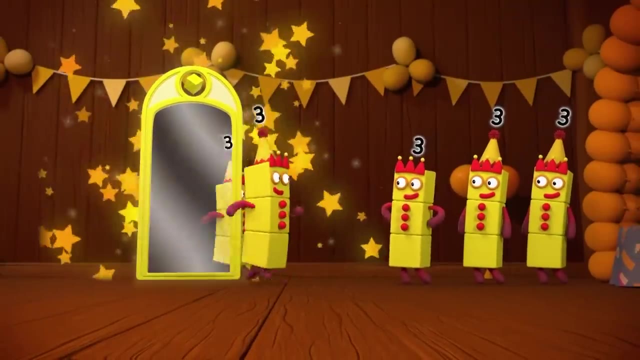 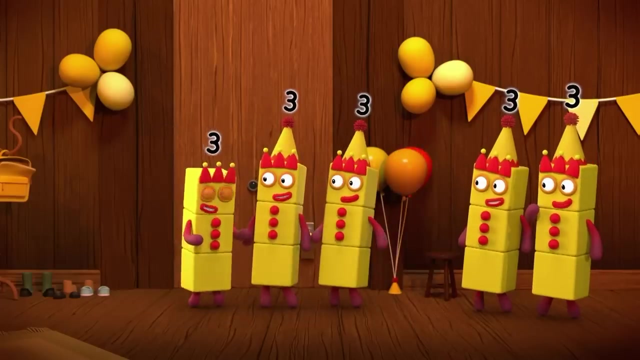 It's just you and me. Good, remember, Don't let three In. Come back here, you. I've got a plan: We make one more three, And then We can just walk out the door disguised as Five. threes are Fifteen. What about us? I know. 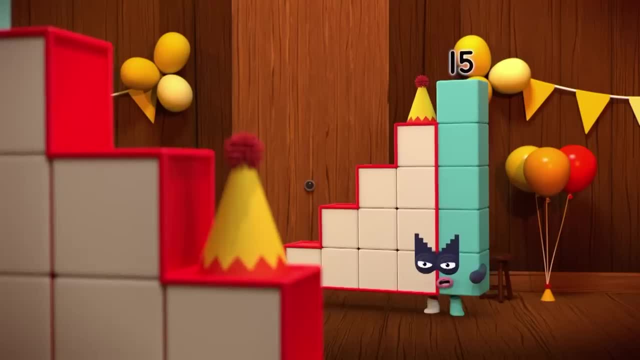 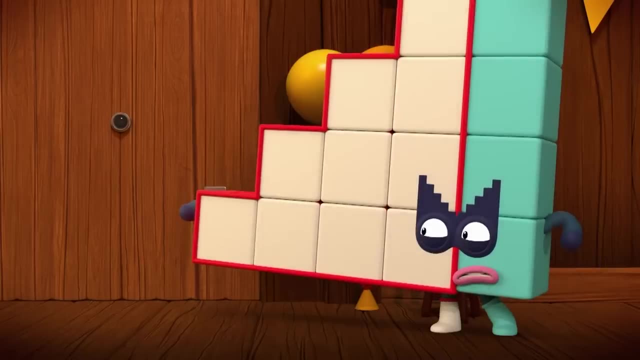 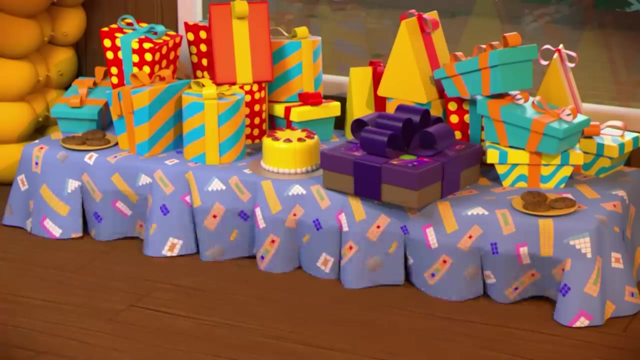 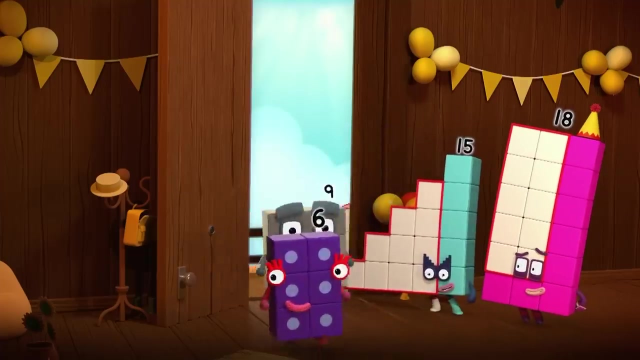 Five, threes are Fifteen. You can't be fifteen, We're Fifteen. The party's in here? Come on everyone. It's fifteen. Everybody hide. Six, threes are Eighteen. There you are, Everyone find a place to hide. When thirty arrives with three, We'll all jump out and say: 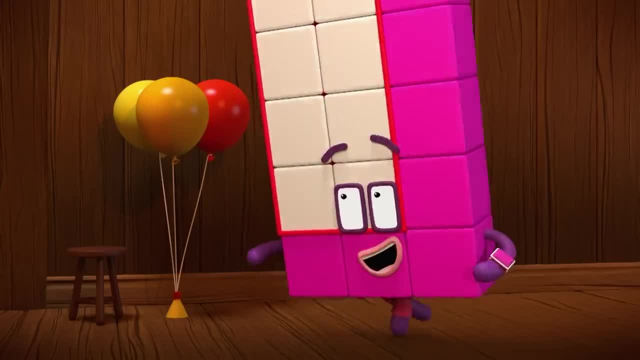 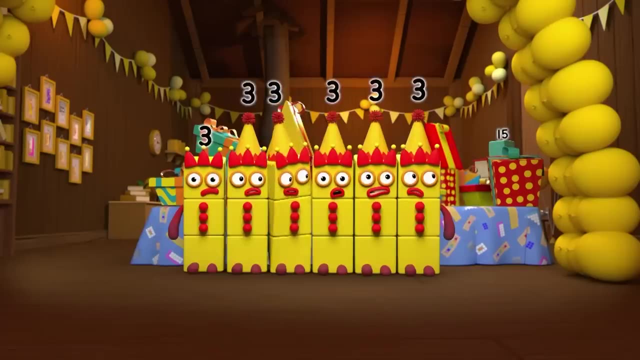 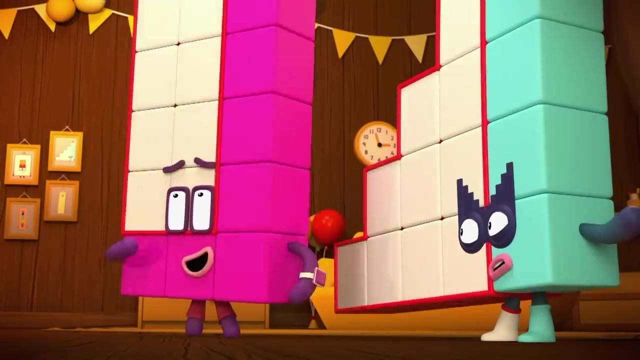 Surprise, Got it. Okie, dokie, dookly, Look, Oh Eighteen, I thought you were here already. Um, No, Seven, threes are Twenty-one. No, just me back here Exploring For a good place to hide. Hope I'm not late, everyone. 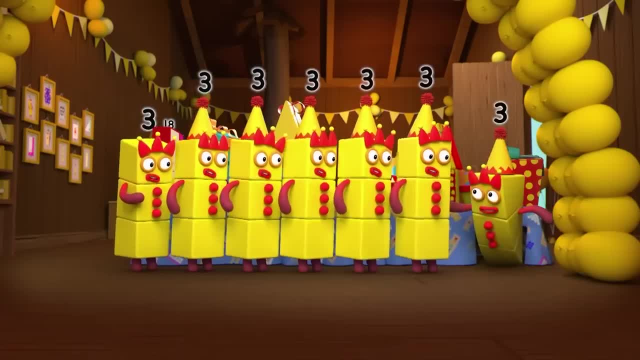 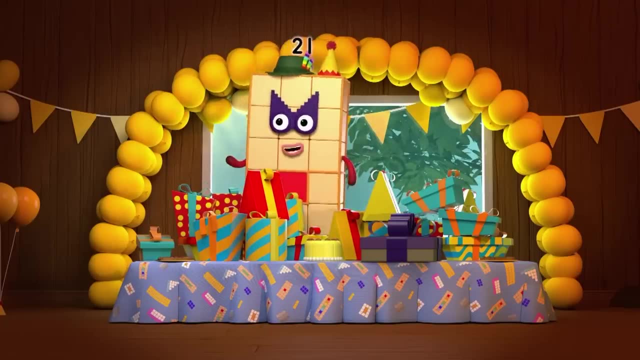 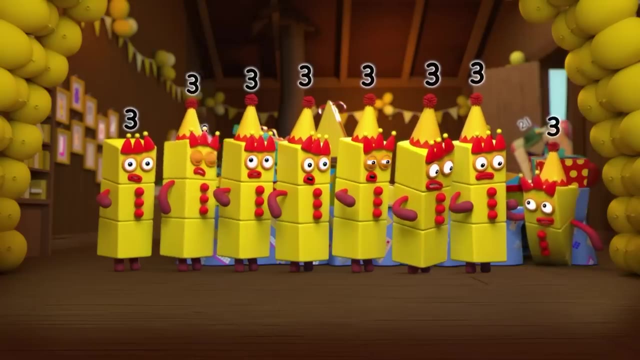 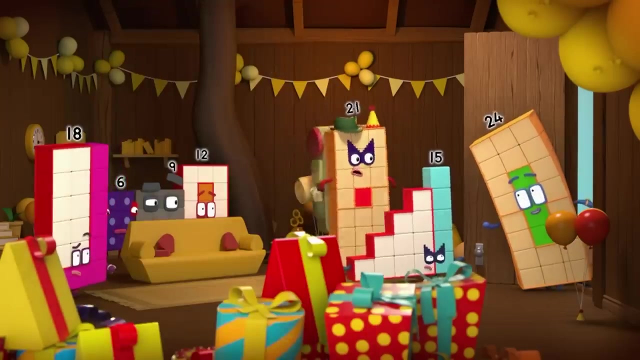 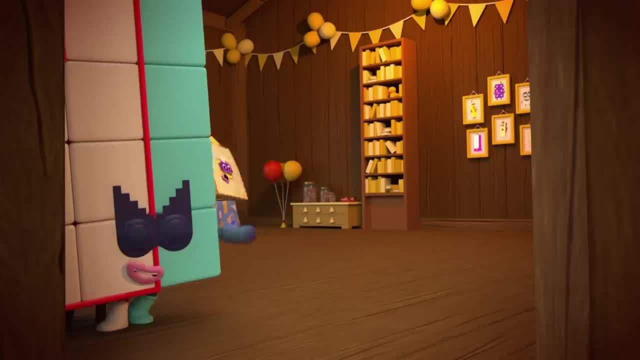 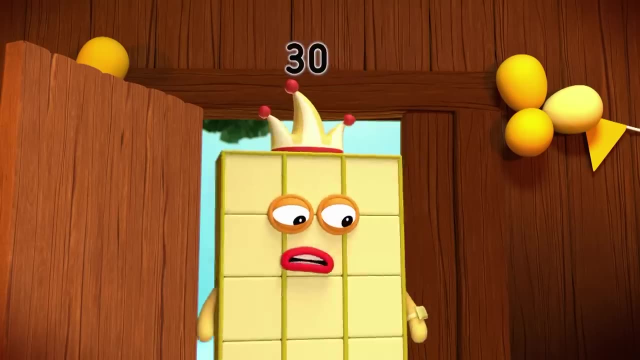 Twenty-four. Gosh, isn't three here, yet It's me Nine, threes, I mean Twenty-seven. Ah, here we are. Is that all of us Need answer Here? I Whoops, Did you say three had gone birdwatching fifteen? 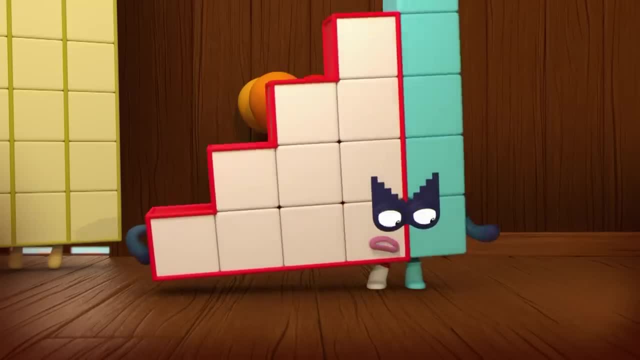 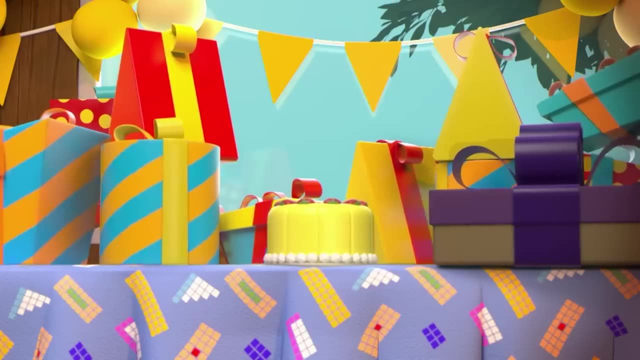 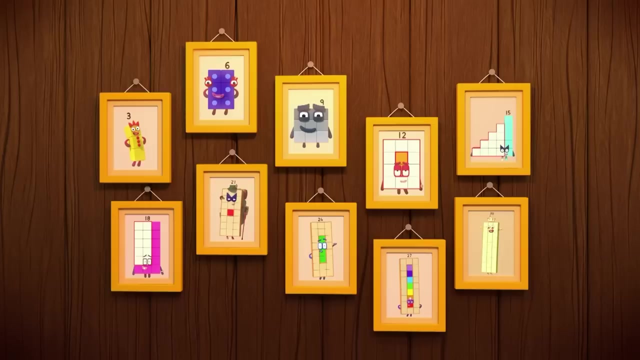 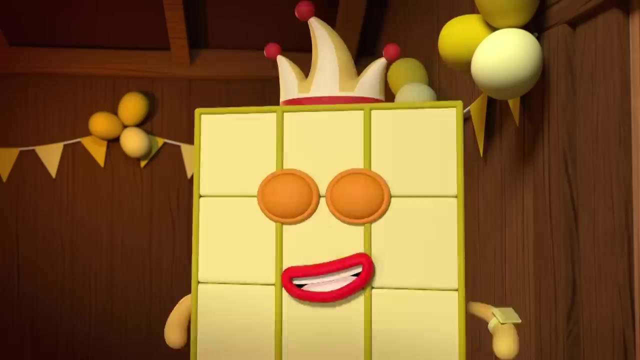 I couldn't find her anywhere. Oh, drat, We can hardly have a surprise party for three without three. Exactly, I've got this. the party is for me, of course. you're the founding member of three club. everyone in three club is made of threes. there'd be no three club without you, the one and only. 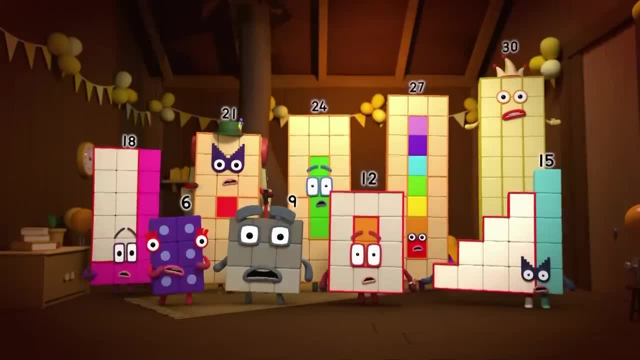 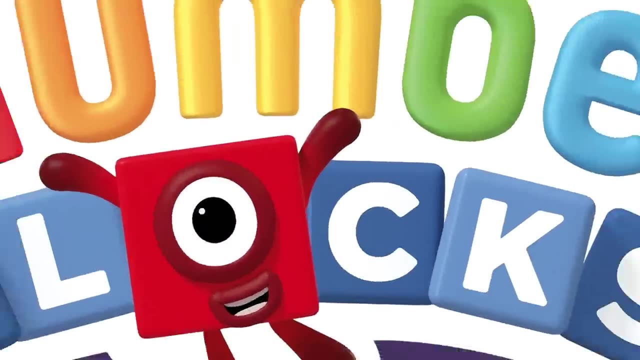 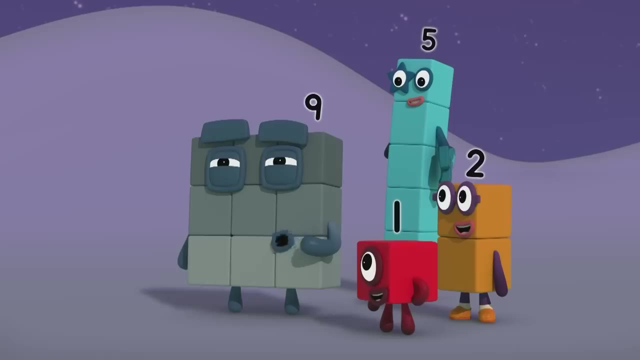 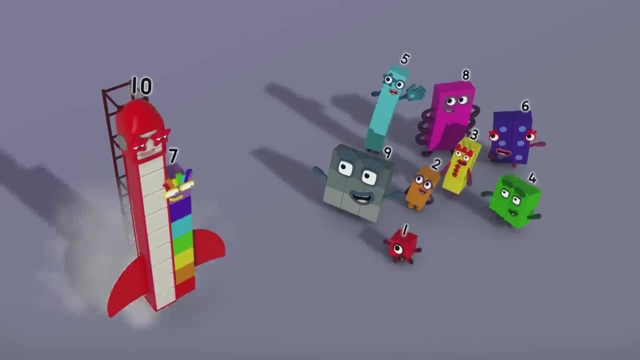 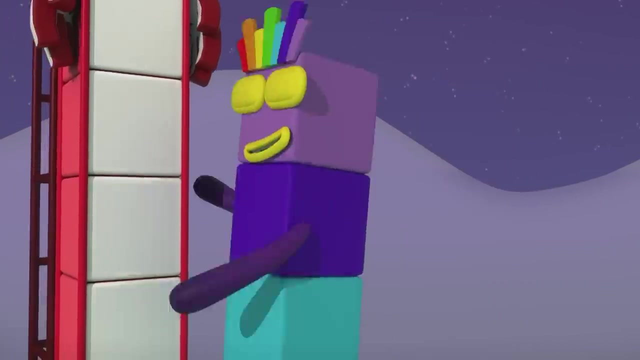 three, surprise ten, threes. i hope the ten gets back here soon. i want to fly up to the moon. ten's rocket rides are really wait for it taking off. we flew to planet seven, where the skies are made of rainbows. thank you, thanks, ten. i'm lucky to have a friend like you. 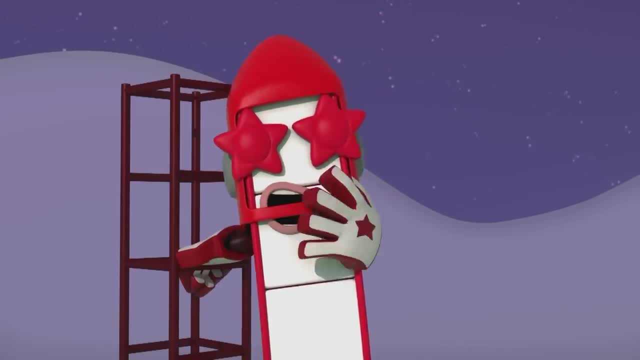 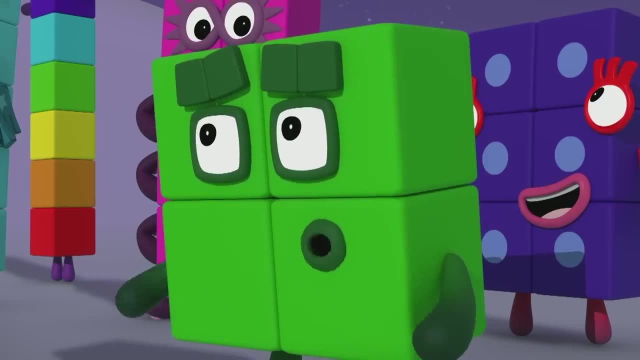 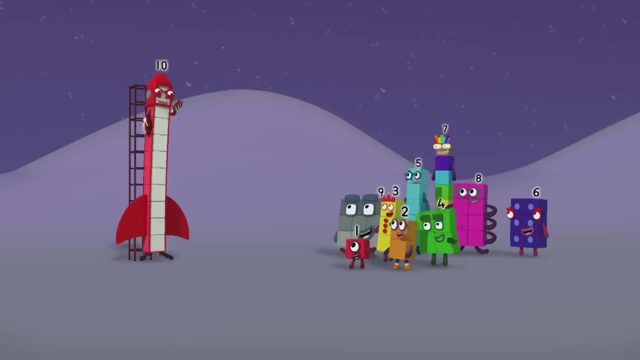 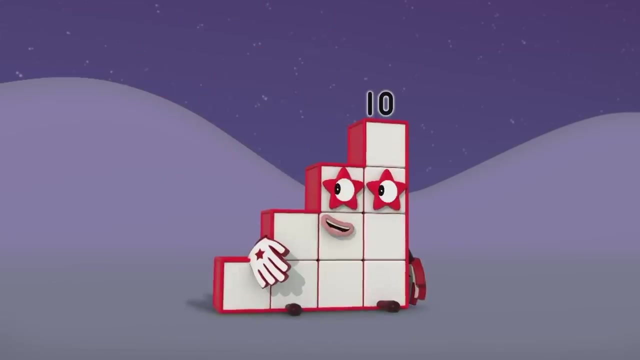 it's my pleasure. seven, so who's next? it's my turn, but only if you're not too tired. what if we all go at once? then it's only one trip. i suppose i can give it a try. oh, blast off, i need a rest. no more rocket rides for a while. this feels like a job for. 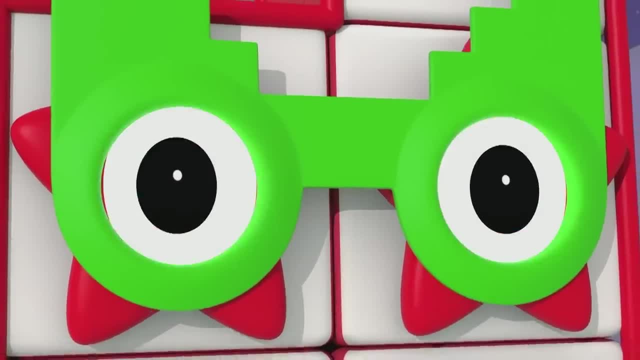 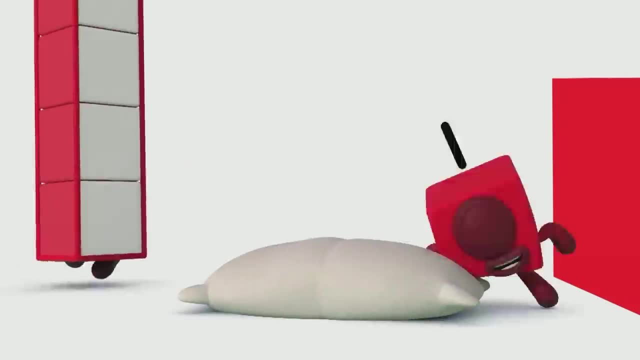 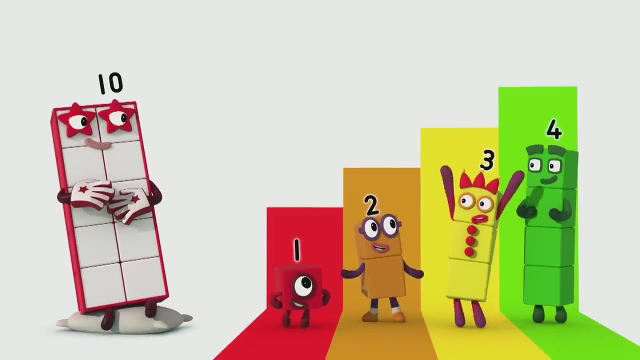 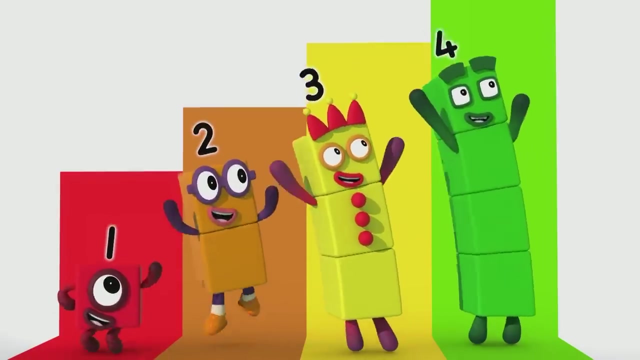 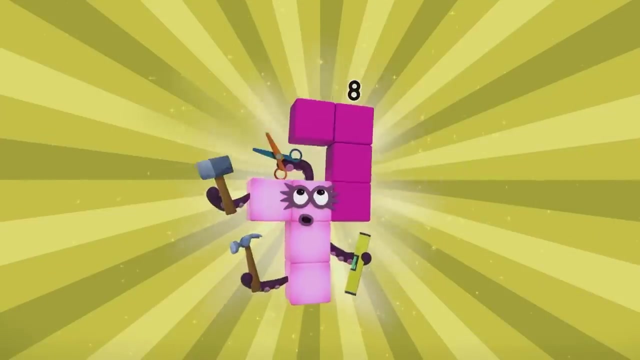 step squad 10 with a four-step plan to reach the stars. step one: let ten, have a nice sit down. step two: build more rocket towers. step three: build more rockets. step four: blast off to the stars. yay, great plan. leave the towers to me. octoblock: build one, two, three, four, five, six, seven, eight, build. 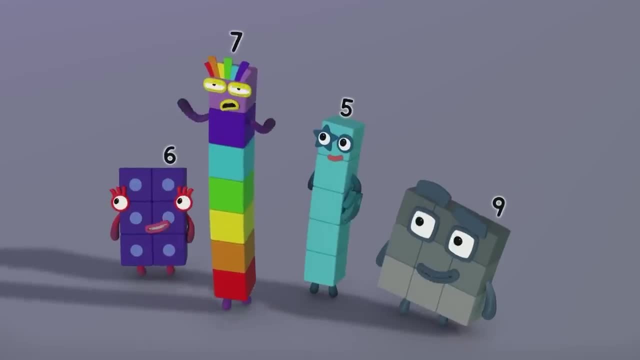 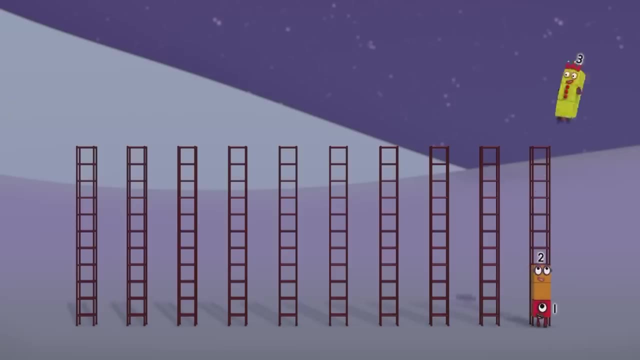 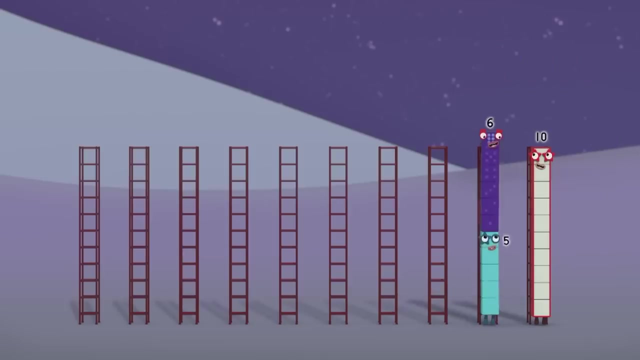 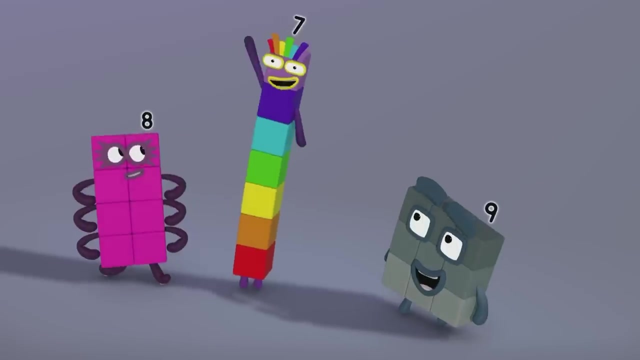 oh there, friend, that should be plenty. now let's make rockets. one plus two plus three plus four is ten, five you're next. five plus six leaves one block in there. I've hit the sky out the frame. i'll slide it down and start again. one me next. one plus seven is eight plus eight is 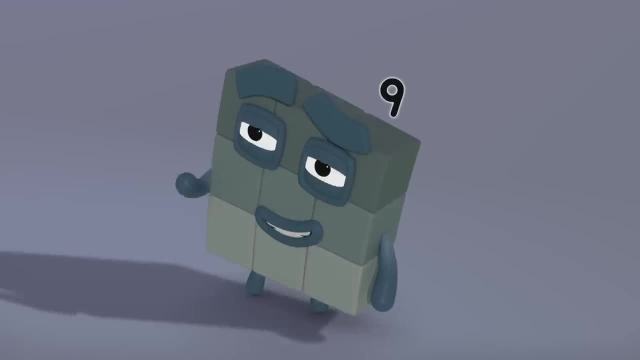 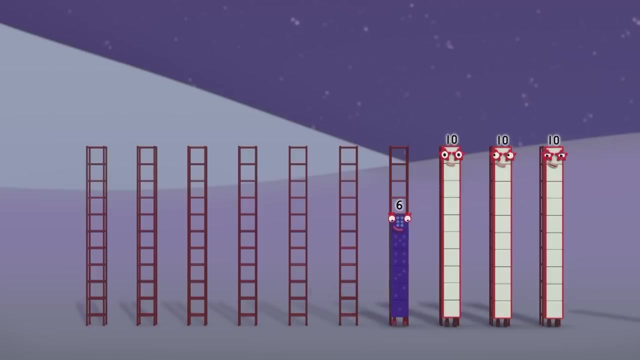 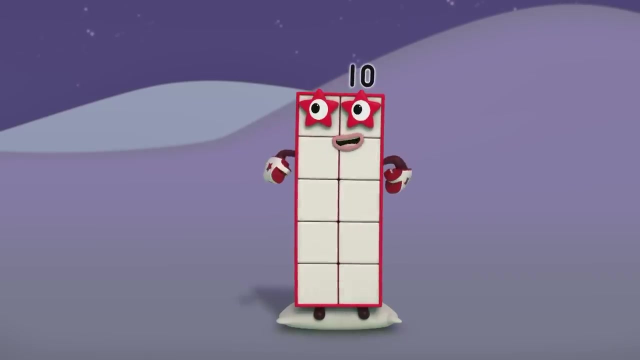 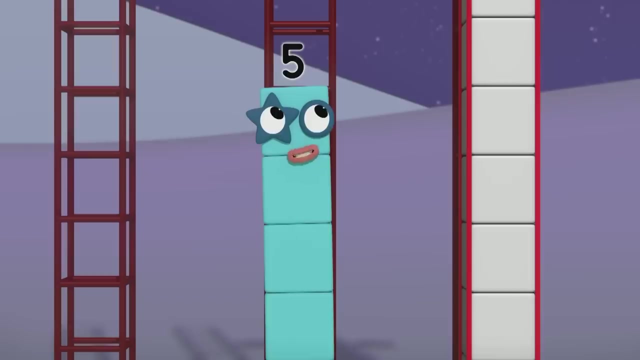 much too tall. you've got six blocks sticking out the top. slide them down for the next rocket. six plus nine is ten plus five. my turn. i'm feeling much better. for that rest. yeah, five plus ten is ten and five. would you look at that? five rockets with five blocks left over. 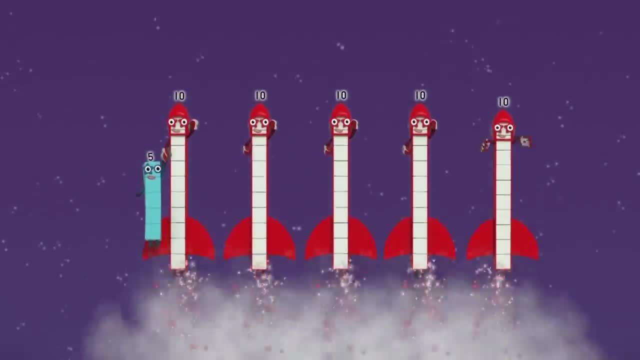 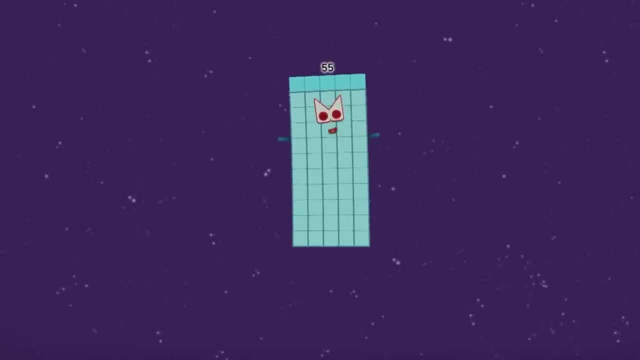 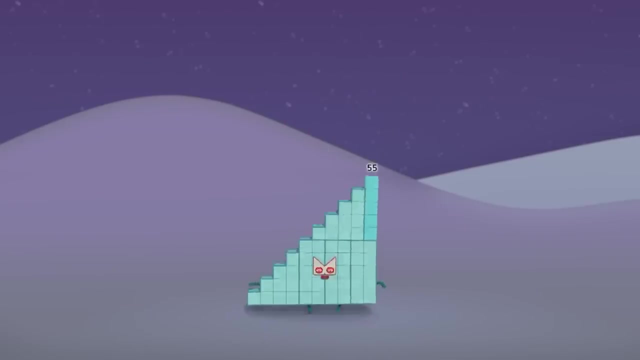 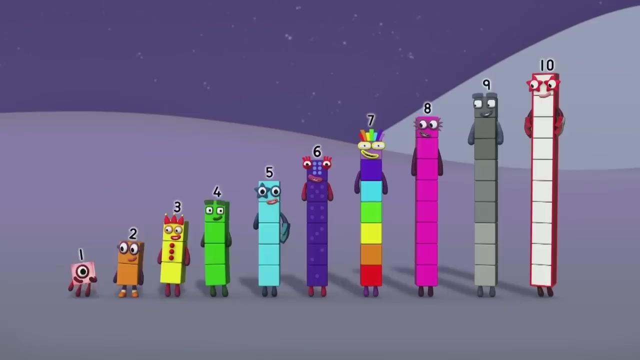 put us together. what have you got? ten, twenty, thirty, forty, fifty, fifty five: the start of the starship explorer, my ten-step mission to step boldly where no number block has stepped before. wow, how lucky is that we all happen to add up to a step squad. um well, actually think about it.